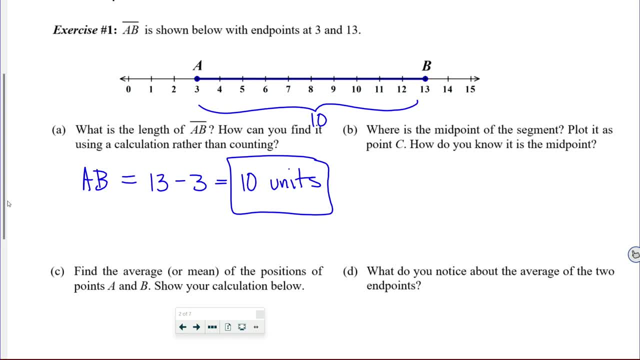 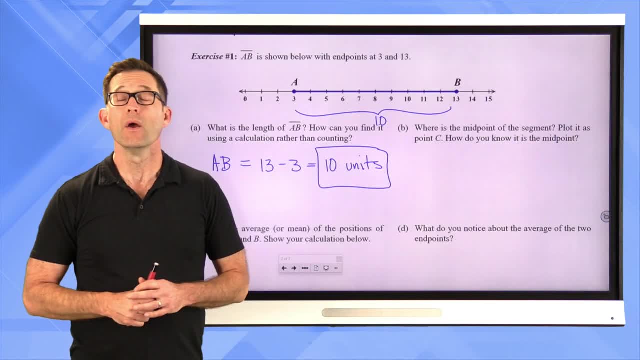 have to count. Let's take a look at letter B. Where's the midpoint of the segment? Plot it as point C. How do you know it's the midpoint? All right, Well, pause the video now and go ahead and figure out where the midpoint is, and then we'll come back to that in a minute. 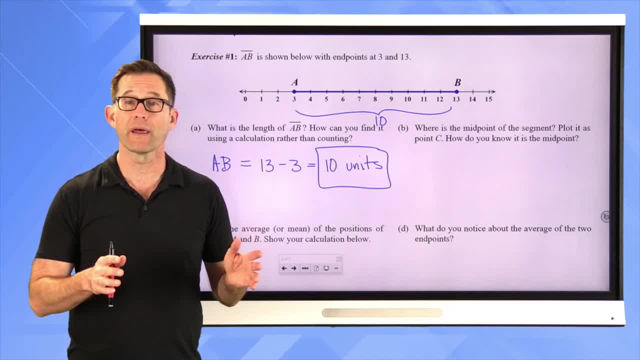 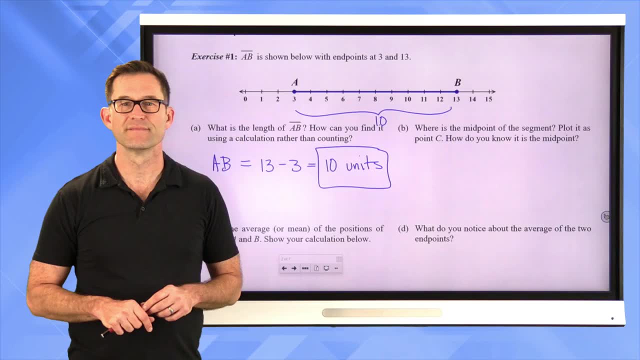 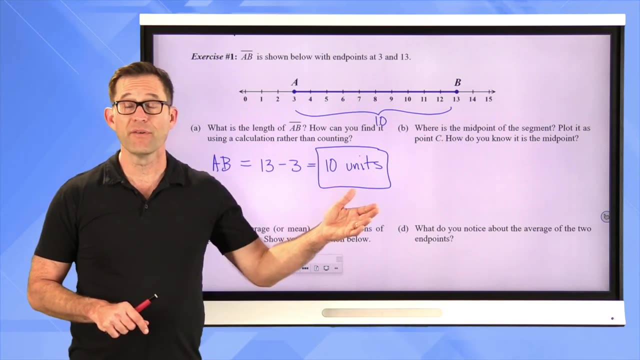 I'm sure that that won't be much of a problem for you Plot it and then how do you know? it's the midpoint, All right. Well, remember, the midpoint is the point that will divide the segment into halves. right, Half of 10 units is 5 units. So if I go 5 units above A or 5 units below B, 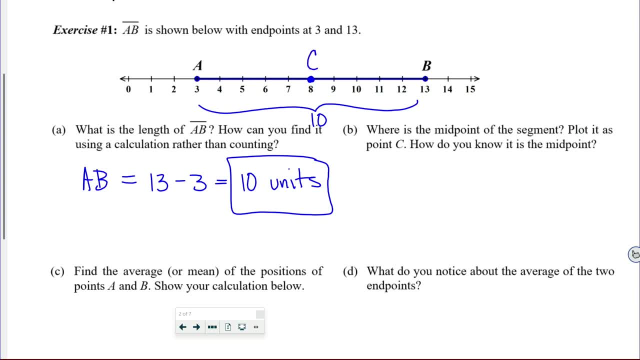 I'm going to be at a place of 8, right. And how do I know it's the midpoint? Well, I know it's the midpoint because AC is 5 and CB is 5, right, And these are equal, All right. 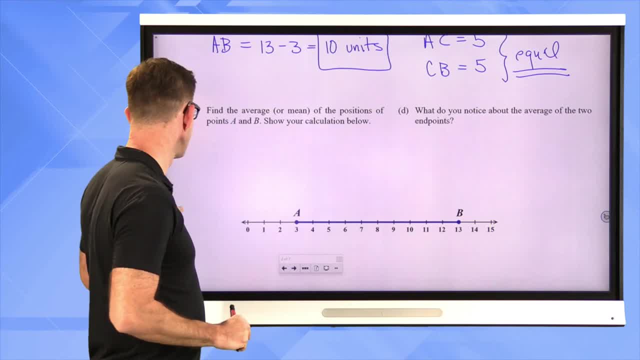 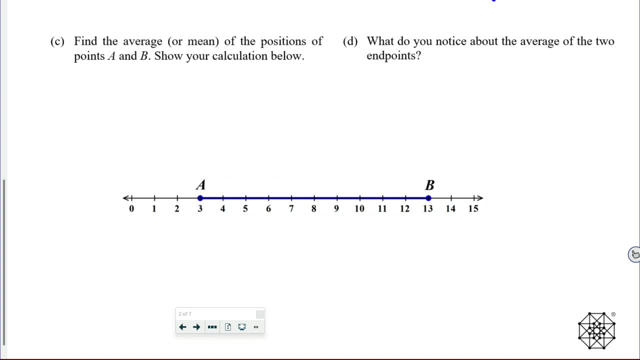 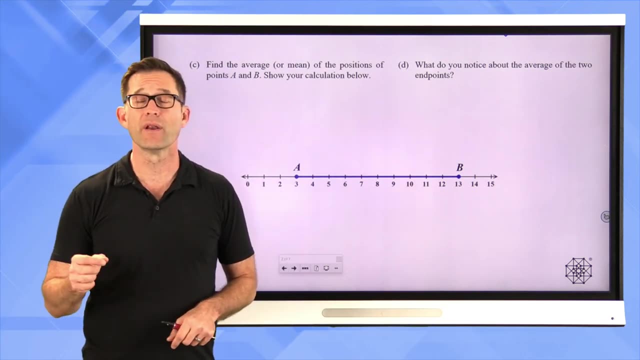 Now let's take a look at letter C. Find the average or the mean of the positions of points A and B. Show your calculation below. All right, So A is at 3, B is at 13,. I just want you to find the average of the numbers 3 and 13.. 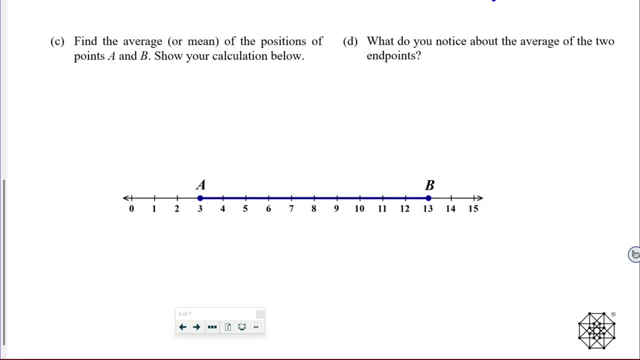 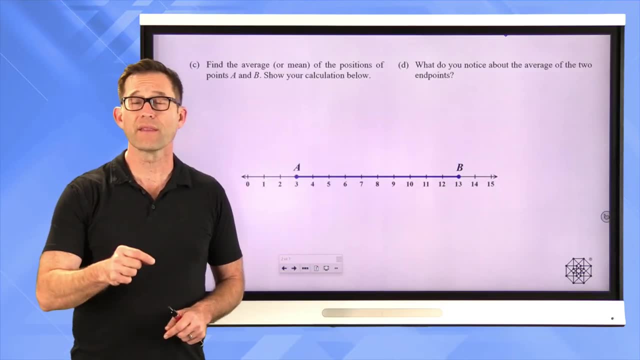 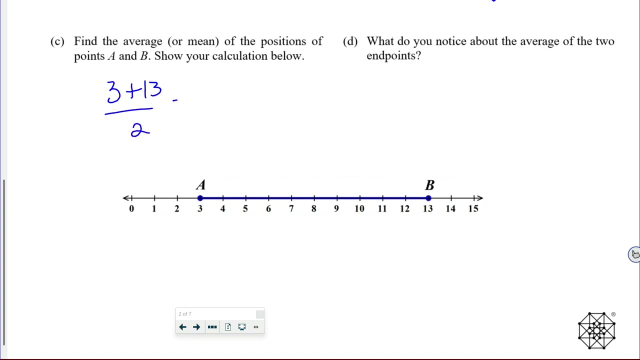 Pause the video now and go ahead and do that. Well, obviously, the average of two numbers, the mean of two numbers, is adding the two numbers together and dividing by 2.. So if I simply do 3 plus 13 and divide it by 2,, 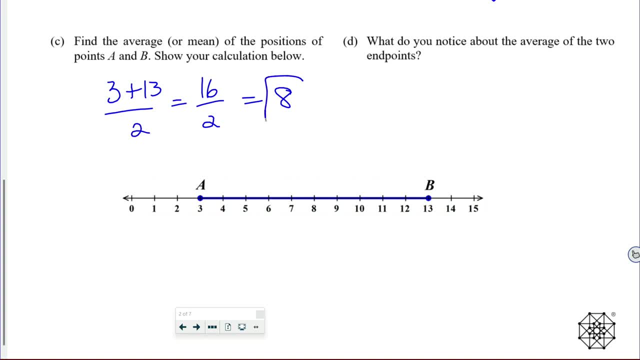 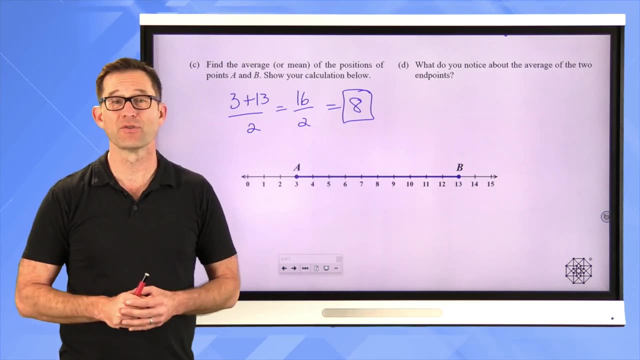 I'll get 16 divided by 2, and I'll get 8.. So the mean of the two numbers is 8.. Now letter D: what do you notice about the average of the two endpoints? Well, hopefully, what you notice about the average of the two endpoints. 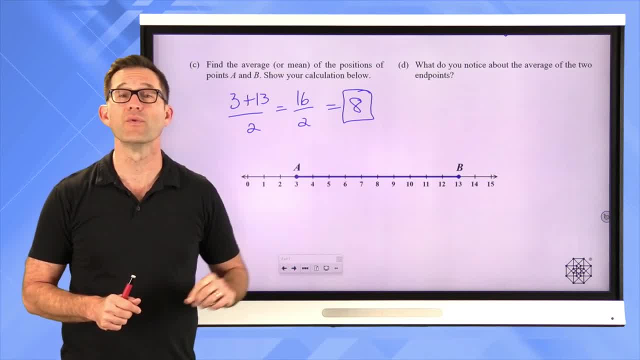 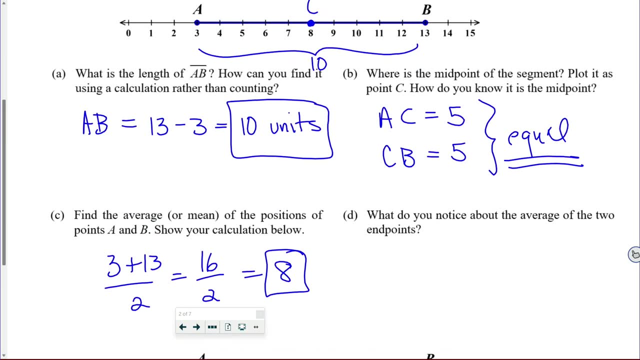 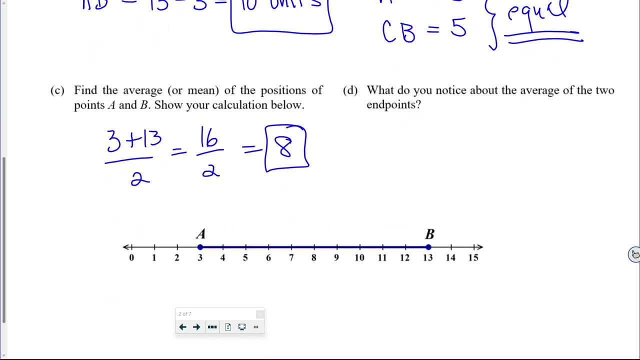 is that it lies at the midpoint or it gives you the midpoint of the line segment Right. Whoops, Here it is right. What did we find? We found that we were at What A midpoint, at 8,. so it is. 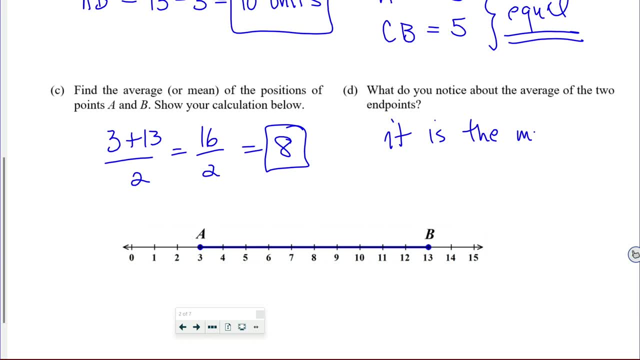 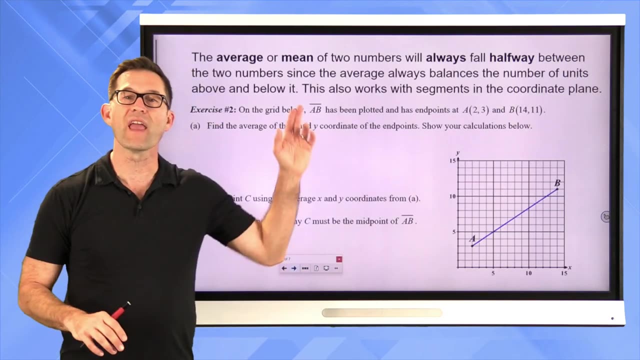 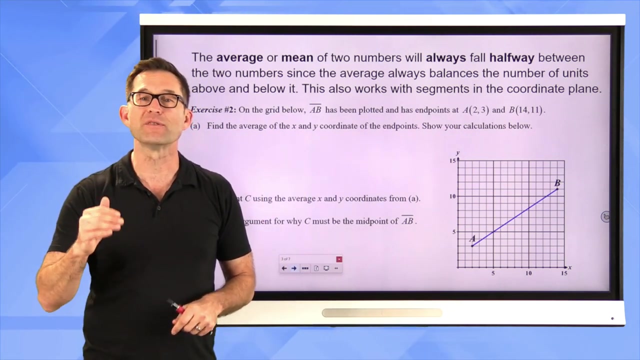 It is the midpoint location, Right, And that should make a lot of sense, right, In fact right. what we should know is that the average, or the mean of two numbers, will always fall halfway between the two numbers, always, Since the average always balances the number of units above it. 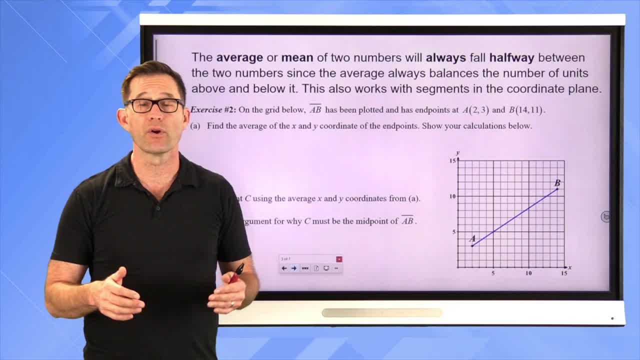 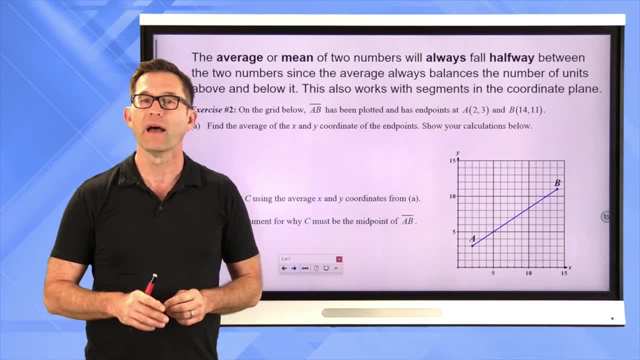 and the number of units below it. And that's true whether or not you're averaging two numbers, three numbers, four numbers or whatever. But in our case we'll only ever be averaging two numbers, And so the amount of distance above the mean. 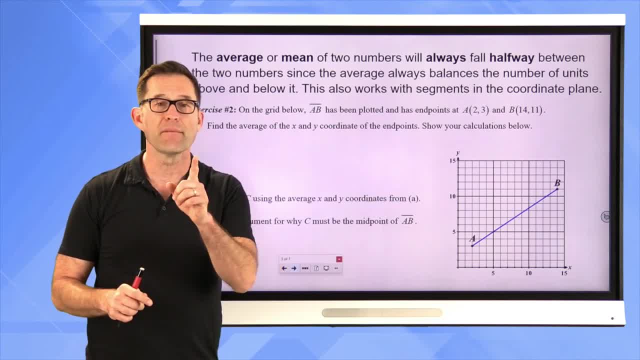 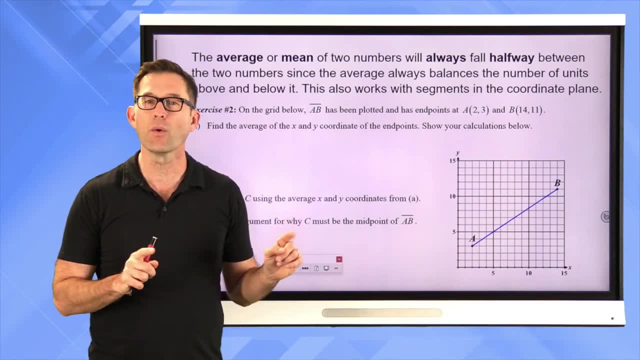 has to be equal to the amount of distance below the mean. That means the mean must be at the midpoint of the two numbers. The cool thing is that this not only works on a simple one-dimensional number line, but it also works with segments in the coordinate plane. 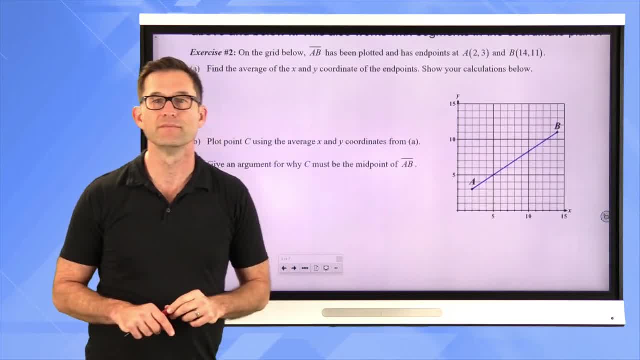 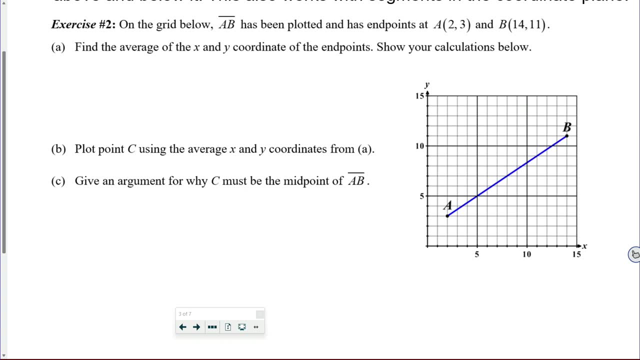 So let's take. Let's take a look at that. in exercise number two, On the grid below, segment AB has been plotted and has endpoints at A, 2, 3, and B 14, 11. Letter A. 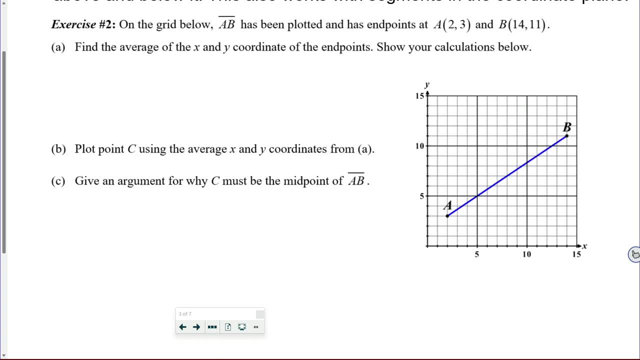 Find the average of the X and Y coordinates of the endpoints. Show your calculations below. All right, Well, let's do the average and the X first. In fact, maybe I'll put X with a little AVG for average down there, Right? 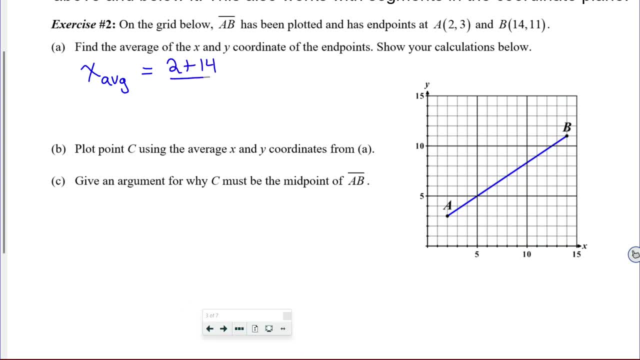 And what would that be? That would be 2.. That would be 2 plus 14 divided by 2, which would be 16 divided by 2, and there's 8 again. Complete coincidence, 8 won't always be the answer. 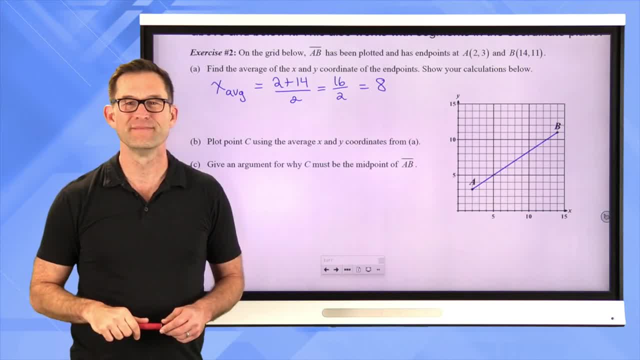 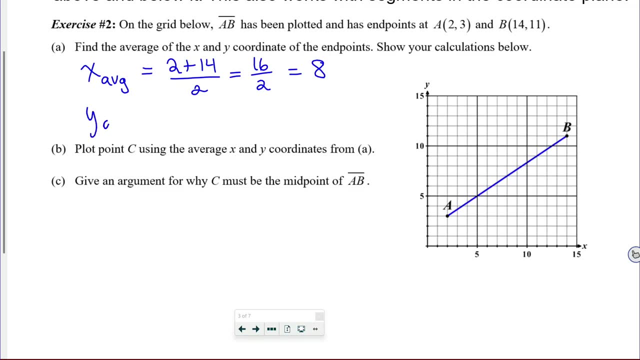 Why don't you find the average of the two Y coordinates All right, That should be simple enough. So Y average, that's going to be 3 plus 11 divided by 2. That's 14 divided That's 7.. 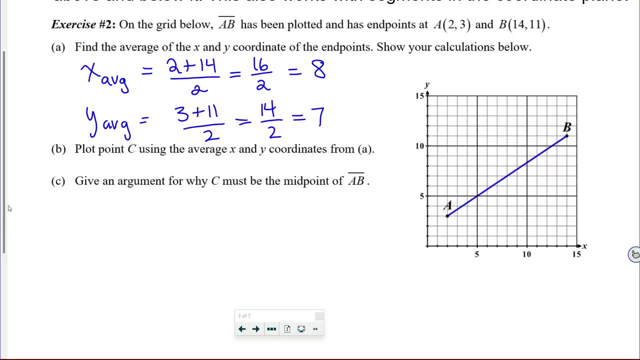 All right, Let's take a look at letter B, Plot point C using the average X and Y coordinates from A. In other words, I want to plot a point of 8, 7.. Let's do that Right. We come over here. 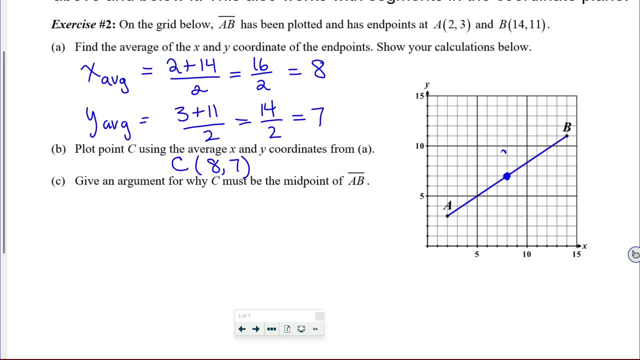 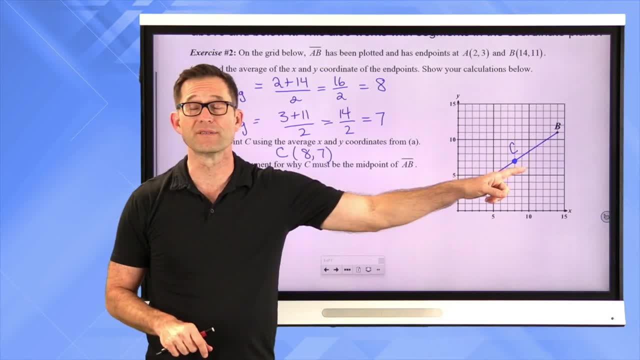 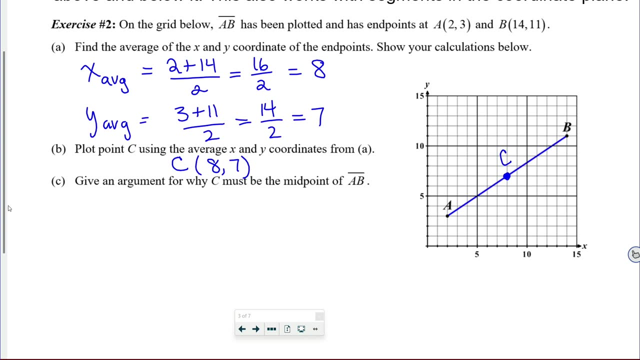 8 up 7.. And we're at point C. All right, Now it definitely looks like point C. Is that right? Point C is the midpoint of AB, right? But let's take a look at letter C Given argument for why C must be the midpoint of AB. 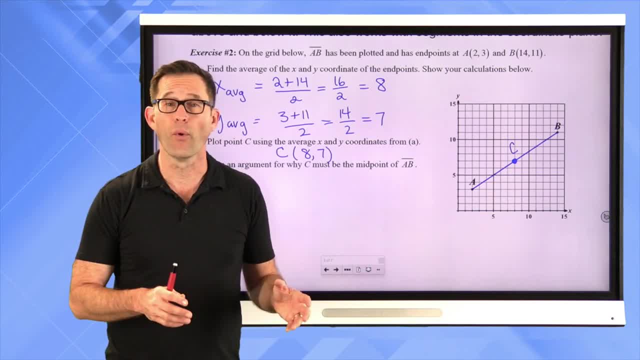 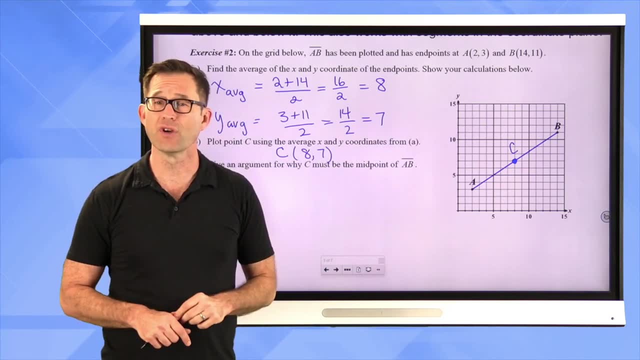 Well, keep in mind, right, that something is going to be a midpoint if it produces two segments that are the same length. So really, the most straightforward way of showing that C is in fact the midpoint of AB is to find the length of segment AC. 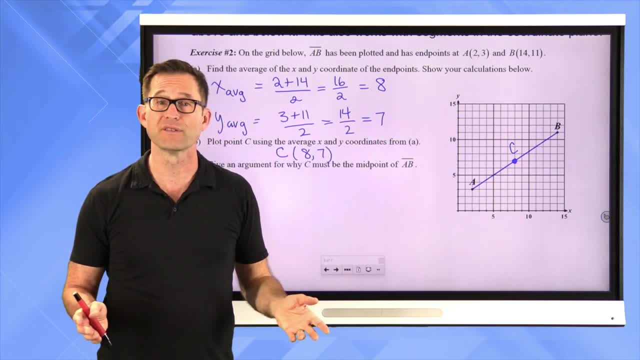 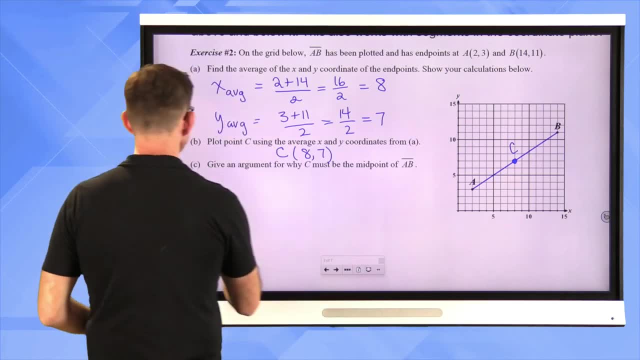 find the length of segment BC and show that they're the same length. How do we find those lengths With the distance formula? So let's do it. Let's find the length of AC together using the distance formula, and then maybe you'll find the length of BC. 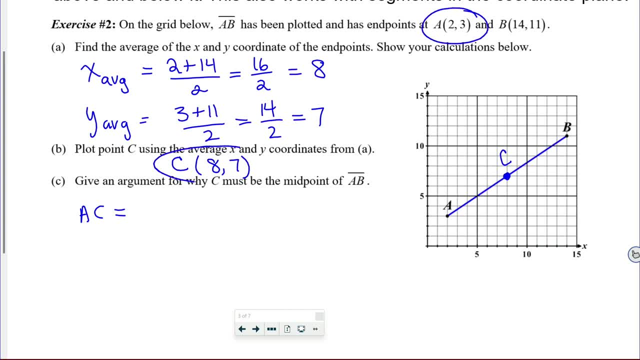 So right. what I'm now doing is I'm now finding the length between A and C Right, And so the distance formula will tell me that I'm going to do 8 minus 2 squared plus 7 minus 3 squared. 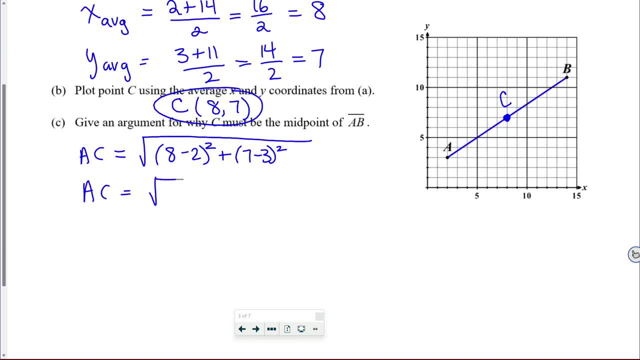 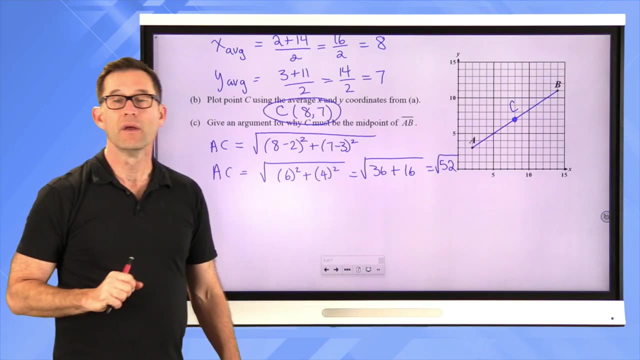 All right. So, taking our time, we'll get 6 squared plus 4 squared. That's going to be 36 plus 16.. And that's going to be the square root of 52.. Now, I don't need to simplify square root of 52 or anything like that. 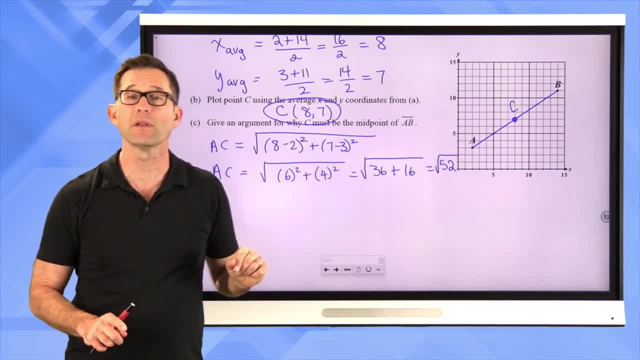 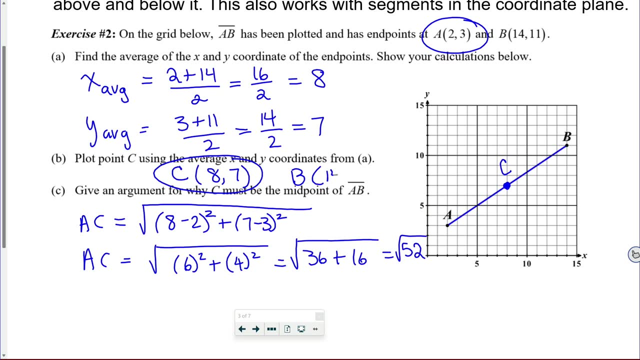 I just want to verify that BC has the same length. Same length. Now, just to be clear about that, maybe I'll put B Right here, That's 14 comma 11.. Maybe I should have put A right here. I just want to be able to see the points. 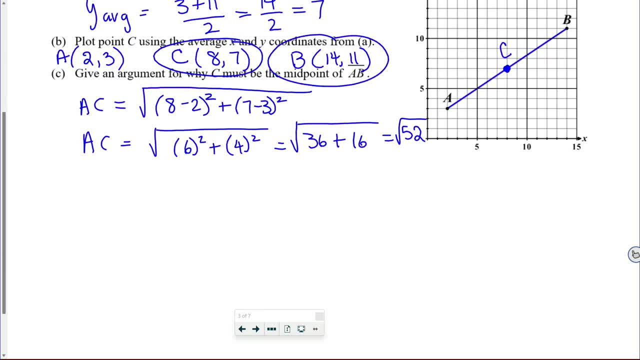 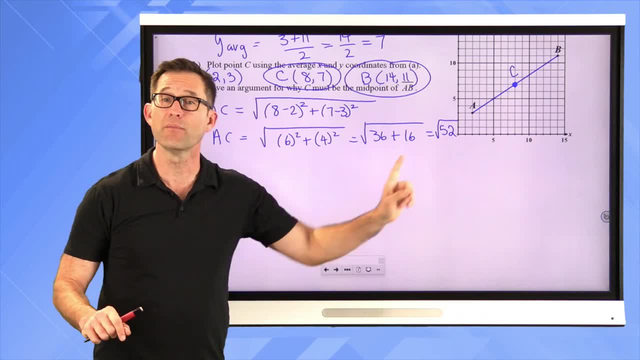 All right. So now what I'd like you to do is calculate the distance between point B and point C. Go ahead and do that right down here. If C is in fact the midpoint, we should also get the square root of 52.. 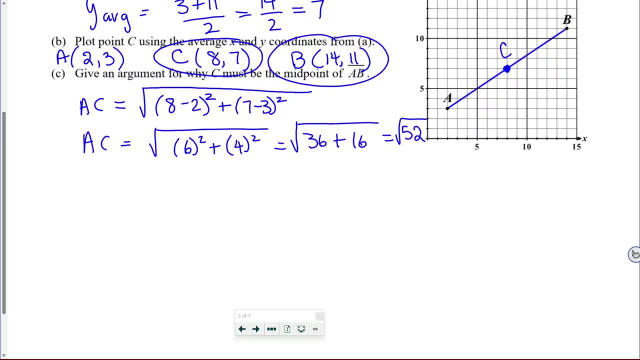 But take a little bit of time to do that, All right. Well, you're going to see right away that it is, But let's go ahead and do that. Let's go ahead and go through it. Right For BC, using the distance formula, we're going to have 14 minus 8 quantity squared. 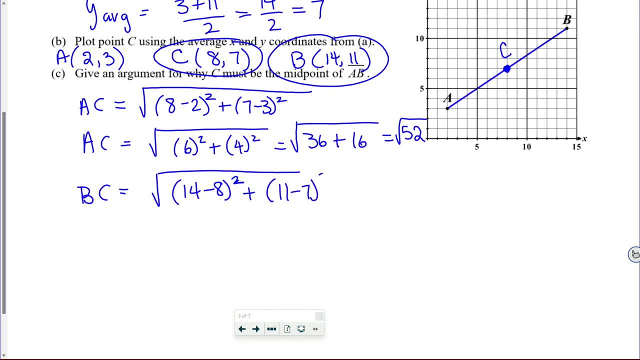 There's a nice squared Plus 11 minus 7 quantity squared. So BC is going to be the square root of 6 squared plus 4 squared, That's the square root of 36 plus 16 again, which is the square root of 52.. 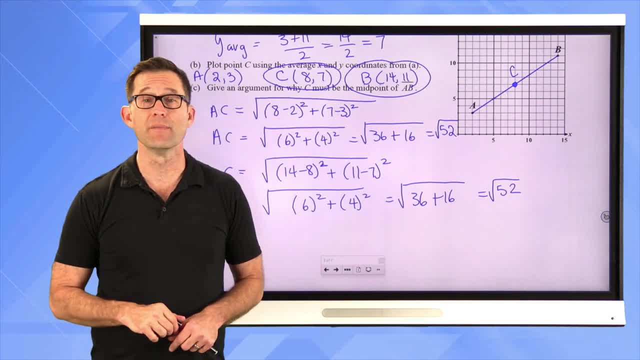 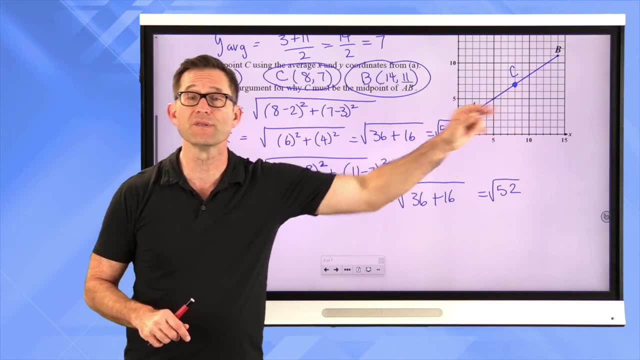 And there it is Right, And that's really all we need to know, that C is the midpoint of AB. In fact, it's the very definition of a midpoint Right. It is a point that divides or partitions a segment into two segments that have the same length. 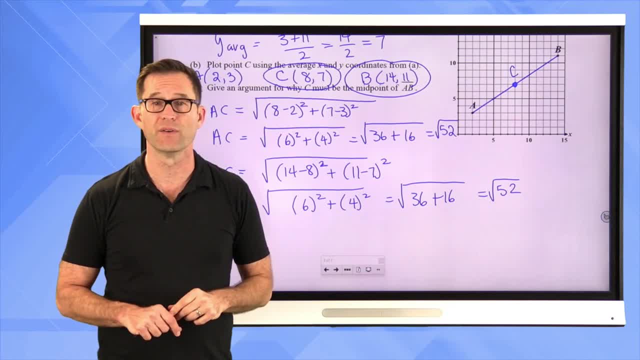 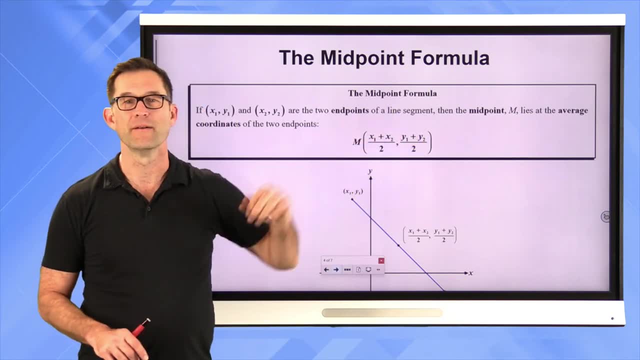 In this case, both of those segments have a length of square root of 52.. All right, So let's formally introduce the midpoint formula now. The midpoint formula If X1 comma Y1 and X2 comma Y2 are the two. 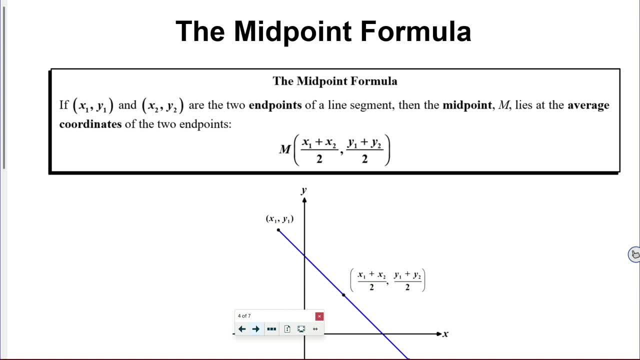 Endpoints of a line segment, then the midpoint M lies at the average coordinates of the two endpoints. In other words, it lies at X1 plus X2 divided by 2 comma, Y1 plus Y2 divided by 2.. All right. 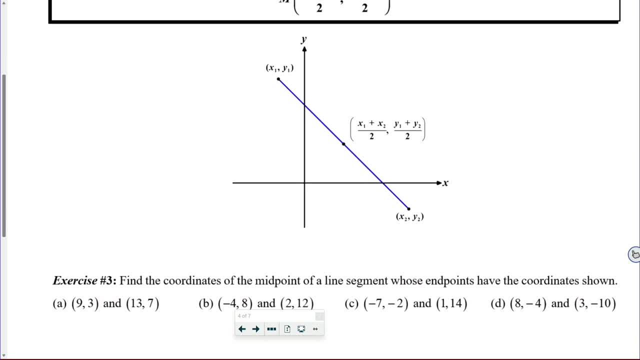 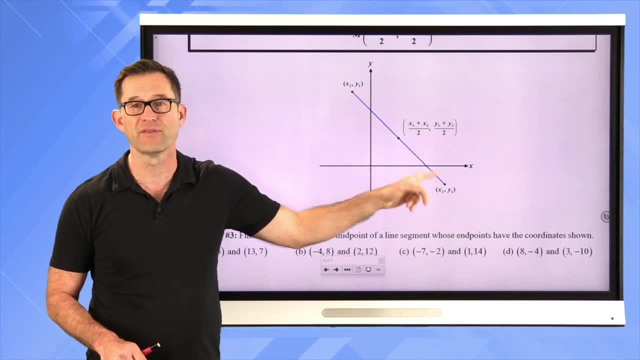 And just kind of illustrating it with this picture. It's very, very simple, Right, I've got X1 comma Y1, X2 comma Y2.. If I want the midpoint, I take my two X coordinates, I average them. 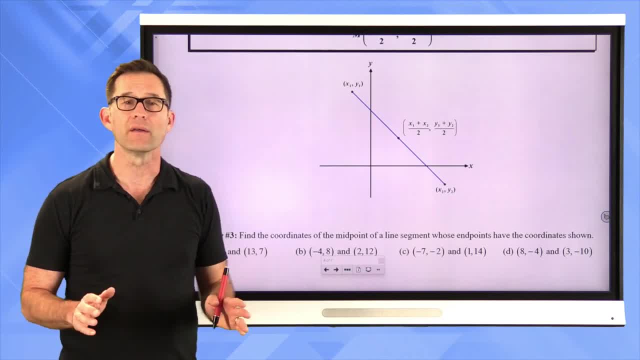 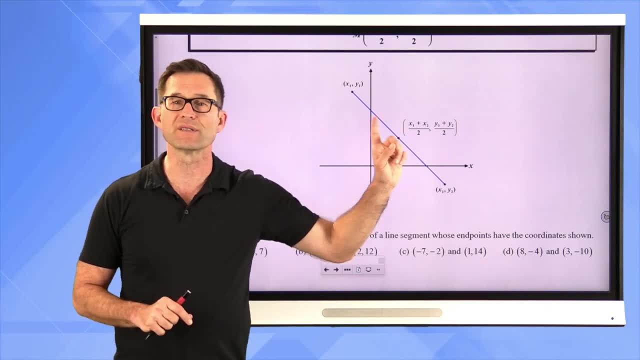 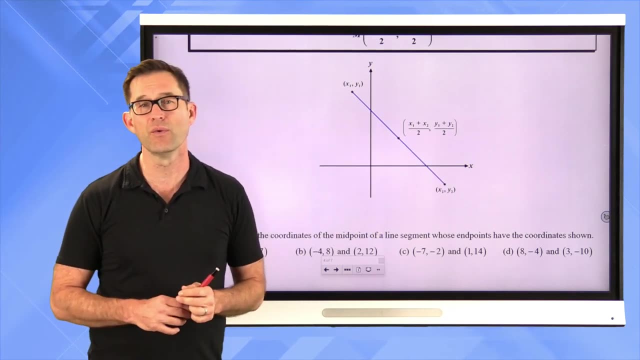 I take my two Y coordinates and average them. The only thing That I have ever found that students find tricky about the midpoint formula is that sometimes they want to subtract the two X coordinates and subtract the two Y coordinates before dividing by two. Now why do students sometimes want to do that? 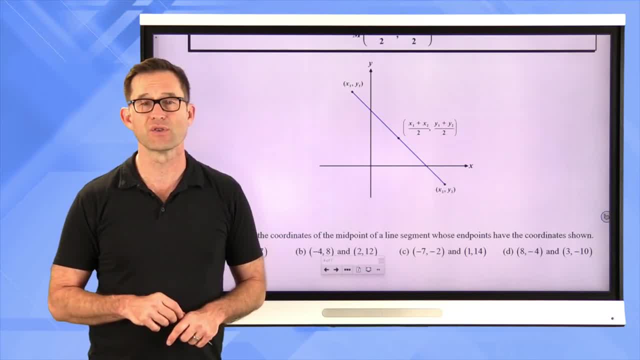 Well notice. the other two important formulas that we've seen in this unit so far have been the slope formula and the distance formula, And in both the slope formula and the distance formula you end up subtracting X coordinates from one another and subtracting Y coordinates from one another. 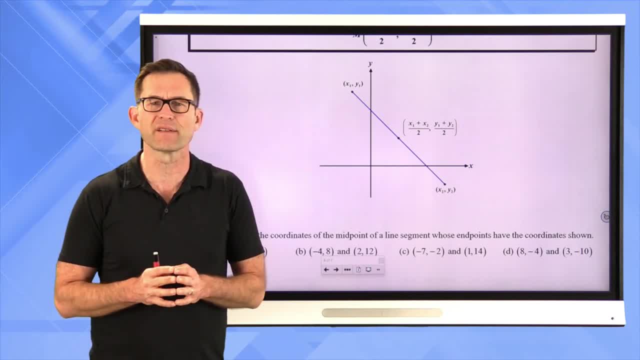 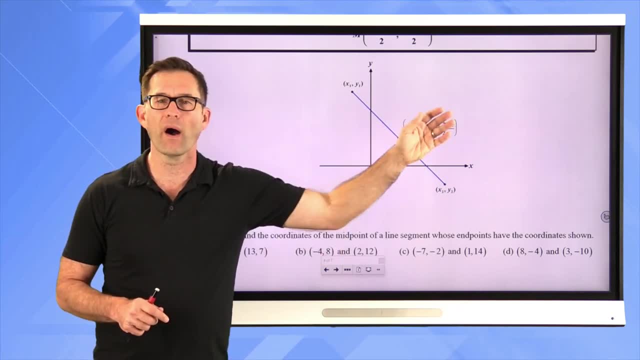 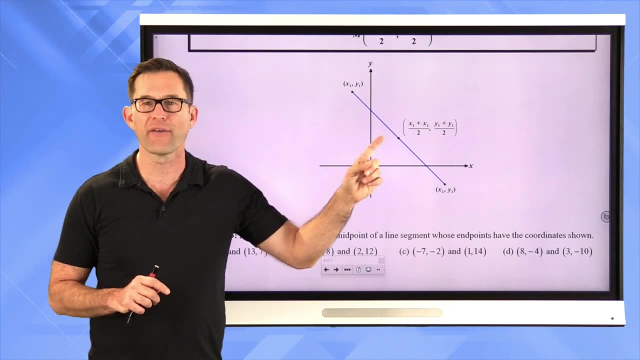 But you're doing that in order to find the distance between the Xs and the distance between the Ys. In this case, we're adding the Xs and dividing by two. adding the Ys and dividing by two because we're trying to find the average X coordinate and the average Y coordinate, which happened to fall halfway between our first, you know, between our two sets of coordinates. 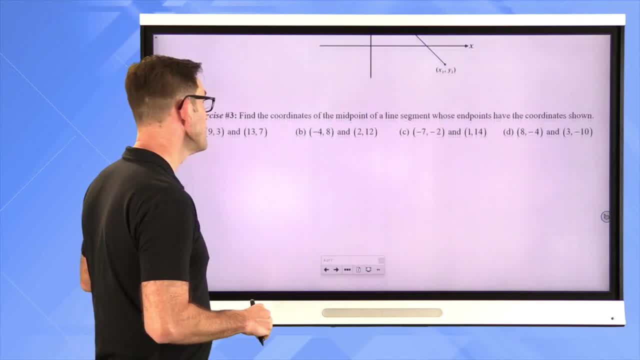 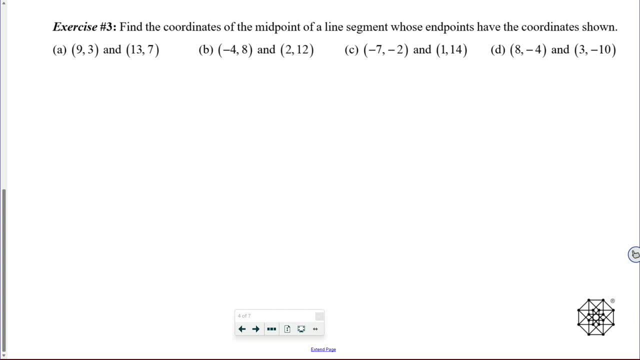 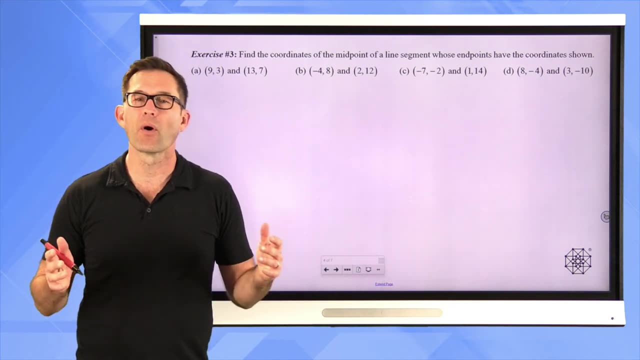 Anyway, it's a pretty darn easy formula to use. Let's use it in exercise three and find a bunch of midpoints. Find the coordinates of the midpoint of a line segment whose endpoints have the coordinates shown. All right, I got four exercises here, but they're all done in the same way. 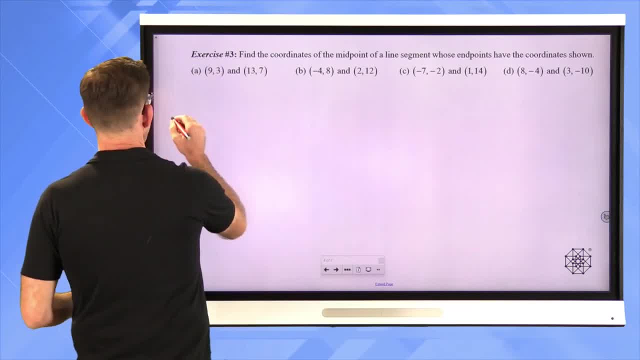 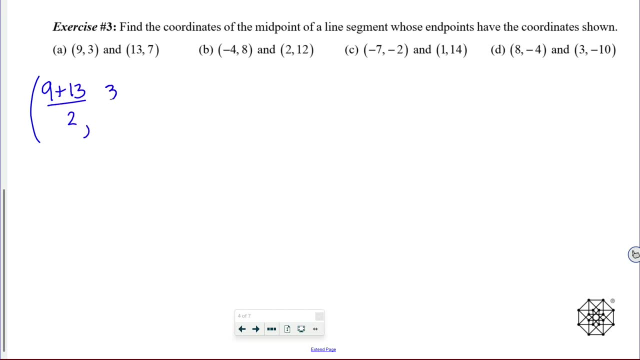 So let's take a look in exercise three, letter A: Right, I want to find the midpoint of this, So I'm going to take the two X coordinates, add them together and divide by two. Take the two Y coordinates, add them together and divide by two. 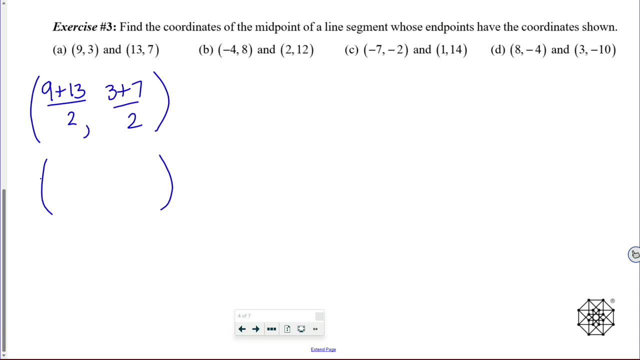 Again, just like all my other formulas, I want to be careful here. Nine plus 13.. 13 is 22 divided by two. three and seven is 10 divided by two. I like it when they end up being even: 22 divided by two is 11,, 10 divided by two is five, and our midpoint is at 11 comma five. 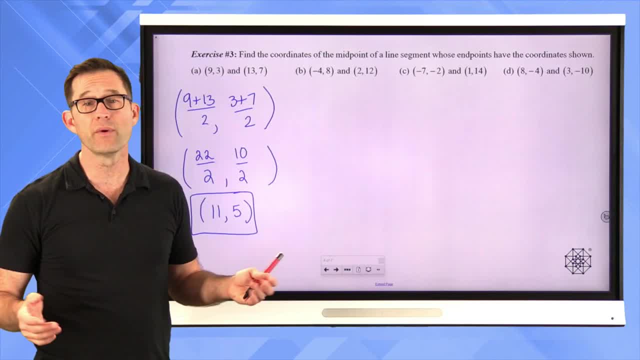 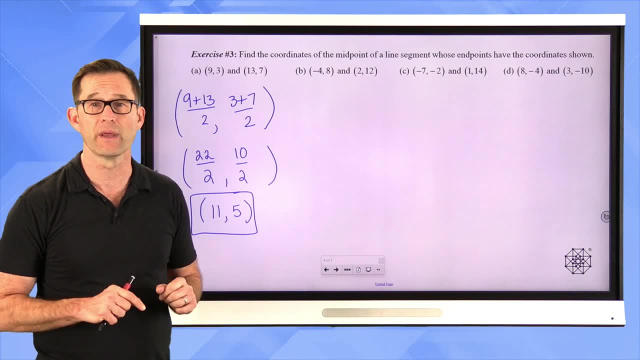 You just can't really get much easier than that, right? Because all I'm doing is finding the average of the Xs and the average of the Ys. That becomes a new coordinate point that is halfway in between. Now, of course, where things can become a little bit dicey is when you have a little bit of time to think about what you're going to do next. 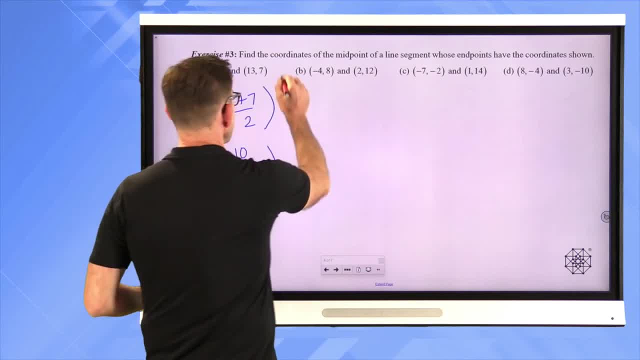 Now, of course, where things can become a little bit dicey is when you have a little bit of time to think about what you're going to do next, When you have negatives involved. let's do one like that, And then I'll have you do B and C on your own. 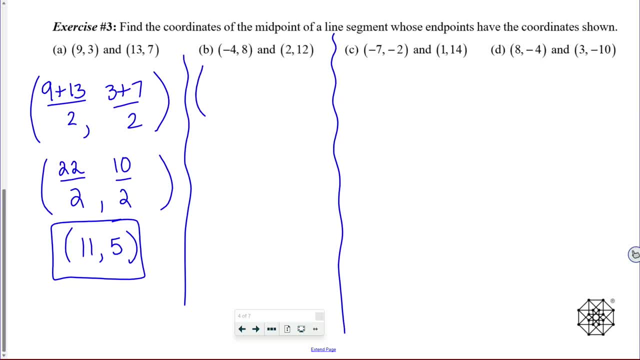 I'm sorry, C and D on your own, So let's do B together. Again, to find the midpoint, I'm going to: take my two Xs, add them together, divide by two. Take my two Ys, add them together, divide by two. 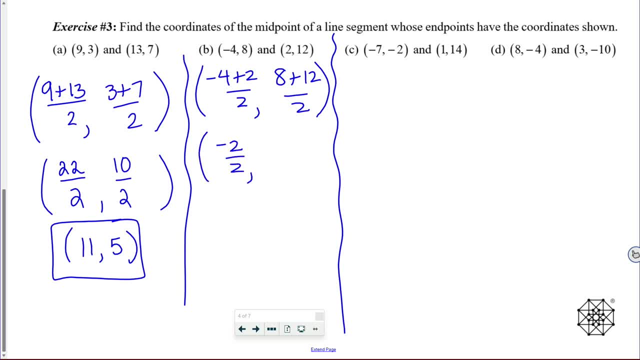 Take my time. negative. four plus two is negative. two divided by two. Eight plus 12 is 20,. divided by two, Negative. two divided by two is negative one. 20 divided by two is 10.. 10, easy peasy lemon squeezy. 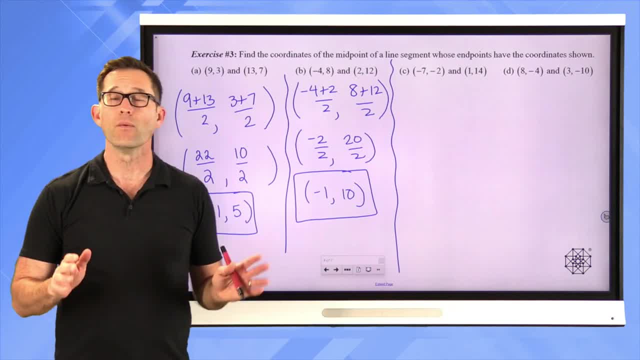 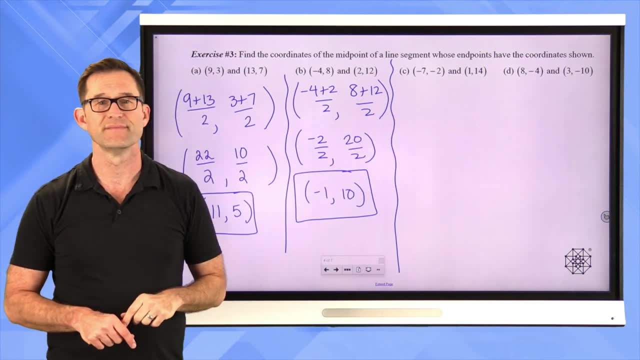 There we go. negative, one comma 10.. All right, what I'd like you to do now is pause the video and go ahead and figure out the midpoint of this segment and the midpoint of that segment. All right, let's do it. 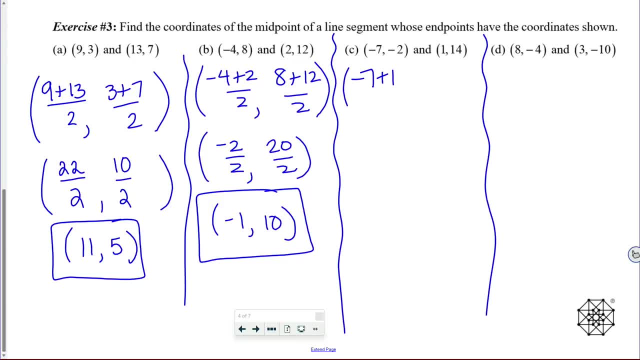 Here we go. Negative seven plus one divided by two. Negative two plus 14 divided by two Negative seven plus one is negative six. Negative two plus 14 is positive 12.. Negative six divided by two is negative three And 12 divided by two is six. 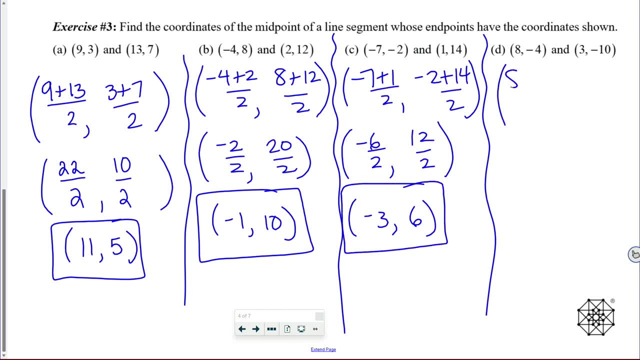 All right for letter D. this is probably the hardest one here, because it's going to have a decimal involved. Eight plus three divided by two, Negative four plus negative 10 divided by two, Eight plus three is 11.. Oh no, an odd divided by two. 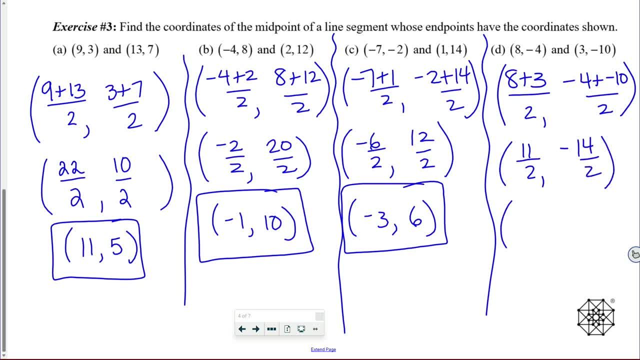 And negative 14.. 14 divided by two- that one's not so bad. 11 divided by two is five and a half or 5.5.. And negative 14 divided by two is negative seven. That's it right. 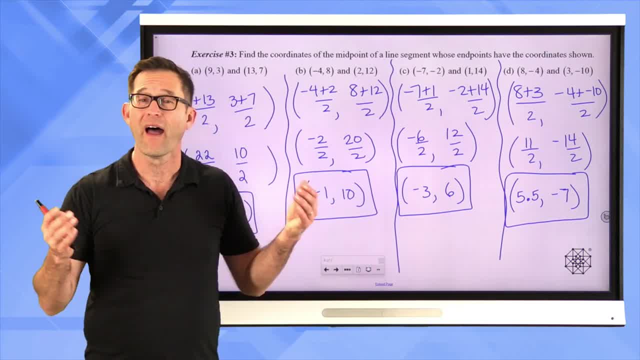 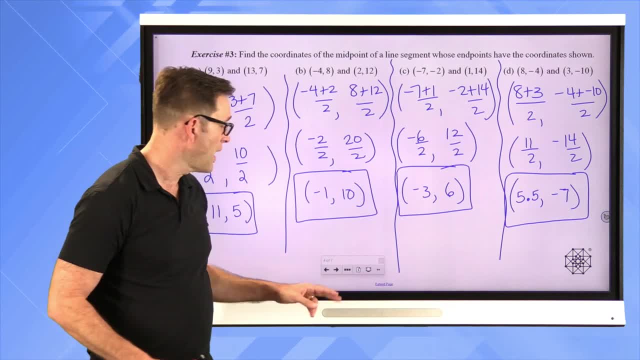 There's not much more to it than that. That is the midpoint formula: Average of the Xs, average of the Ys, and that puts you right in the middle of the two and you have your midpoint. Now we can end up using the midpoint formula quite a bit. 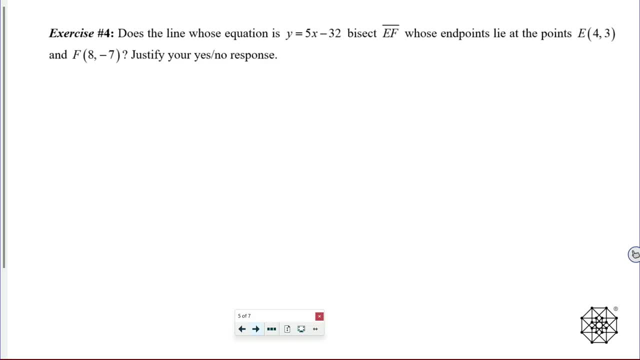 Let's take a look at exercise number four. Let's take a look at exercise number four. Does the line whose equation is Y equals 5X minus 32 bisect segment EF whose endpoints lie at the points E, 4,, 3, and F, 8, negative 7?? 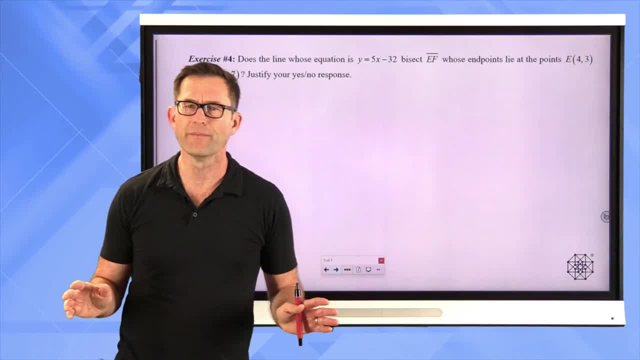 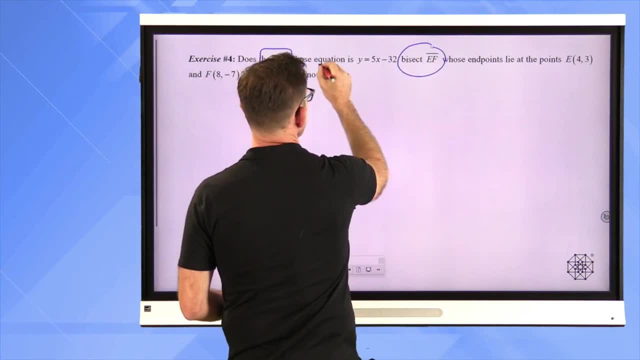 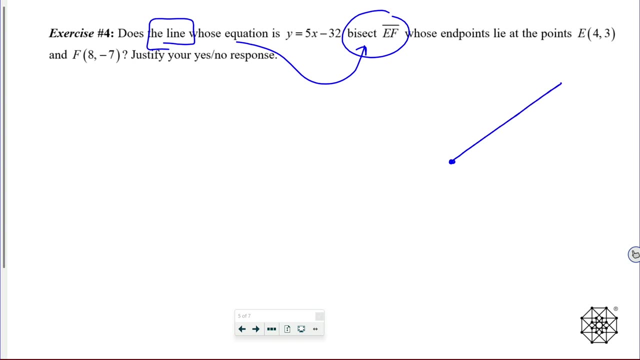 Justify your yes-no response, All right. Well, the first thing that's really important is to understand what it means for a line to bisect a line segment. So just for a minute, right, Like if I had a line segment, right. 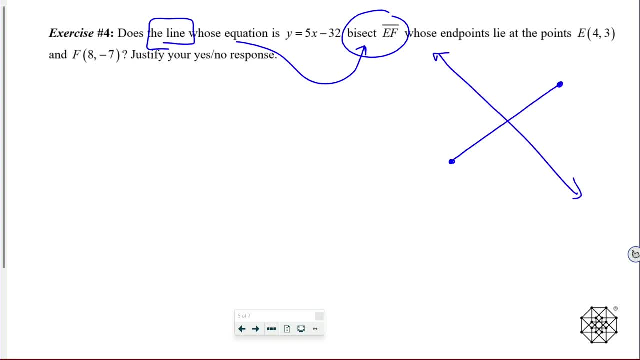 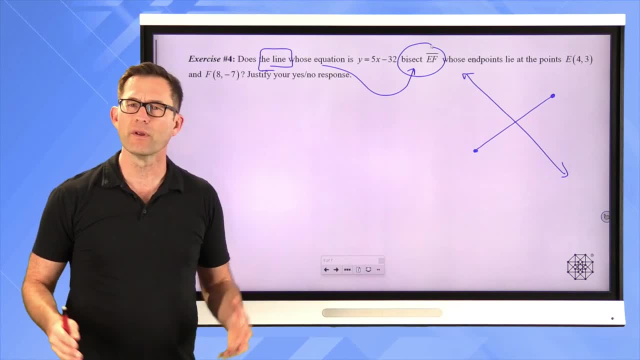 And let's say that I had a line that was bisecting it- And I'm not talking about being a perpendicular bisector, right. I even tried to draw that so that it wasn't perpendicular to the line segment. But what does it really mean, right? 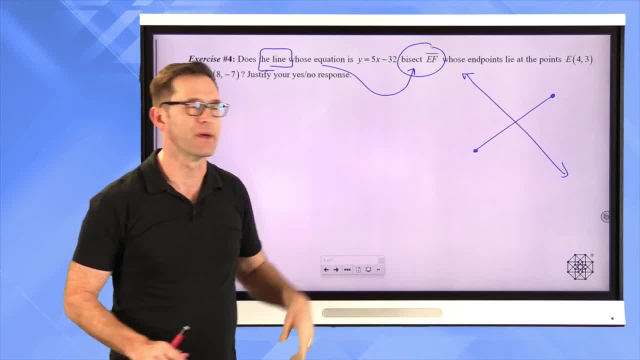 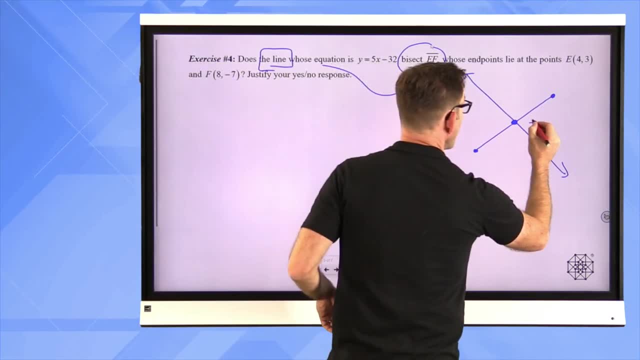 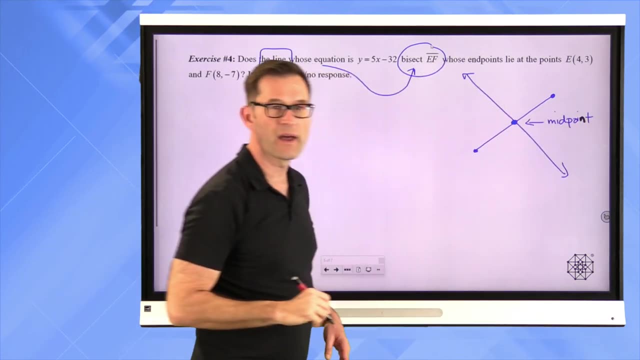 If a line bisects a segment, what that means is that that line goes through the midpoint right of that line segment, Goes through the midpoint Of that line segment. Well, that was interesting. I had a little bit of a black show up this time, instead of red. 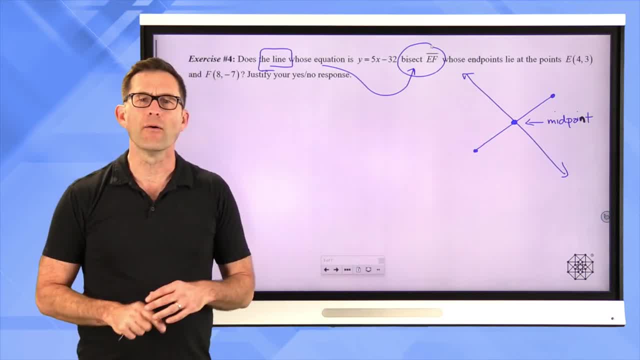 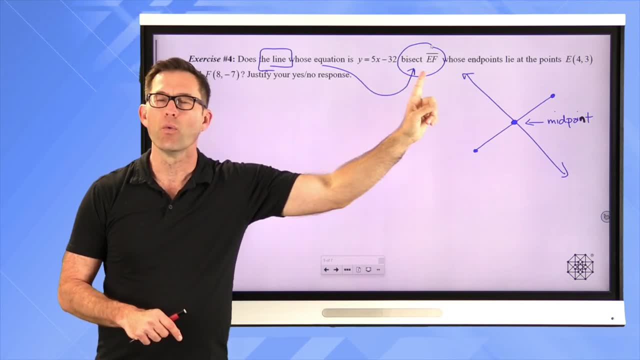 Cool, Okay, So pause the video now and see if you can figure out whether or not a line that has Y equals 5X minus 32 will bisect a segment whose endpoints are given. Pause the video now, See if you can play around with this. 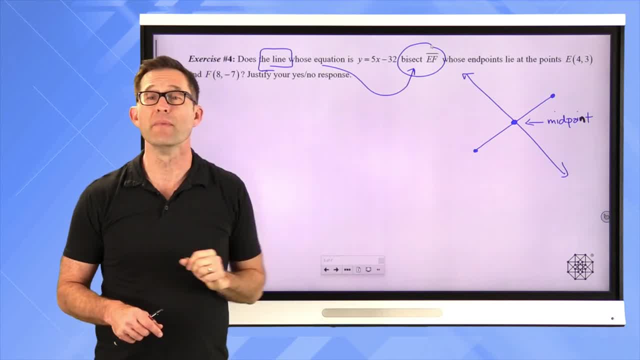 Okay. Well, in order for this line to bisect, To bisect that segment, it's got to go through the midpoint of that segment. So the first thing I'm going to do is figure out the midpoint of segment EF. All right, 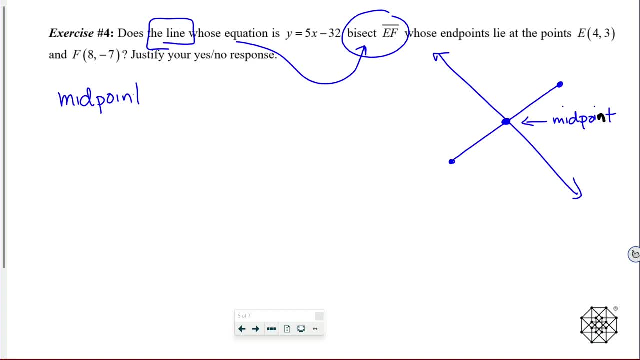 So let me just lay that out, The midpoint of EF. Let's just figure out where that is All right. Well, I can do that by just doing what we just did: Add the two Xs and divide by 2.. 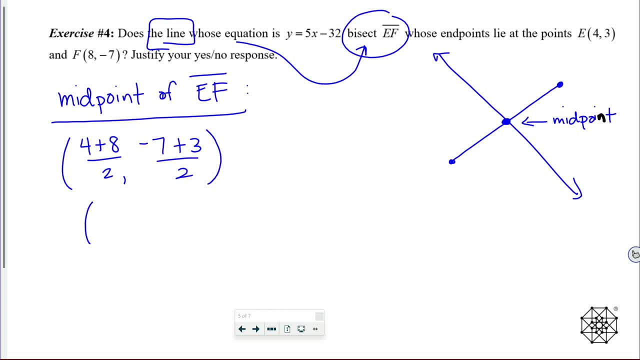 Add the two Ys and divide by 2.. All right, It's going to be 12 divided by 2. And negative 4 divided by 2. And that's going to give me a midpoint at 6 comma negative 2.. 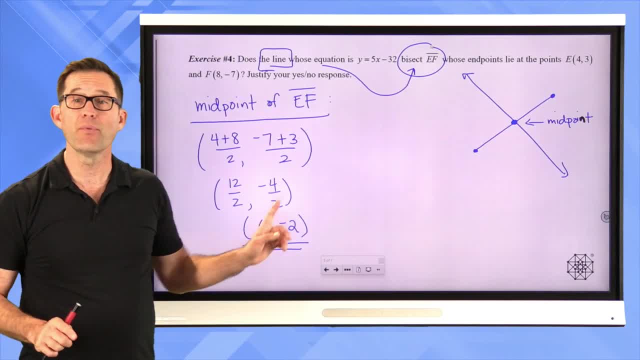 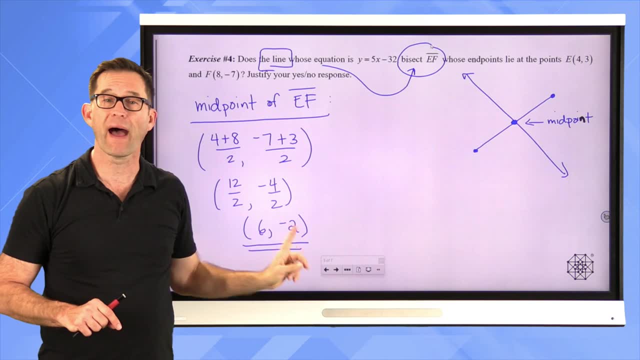 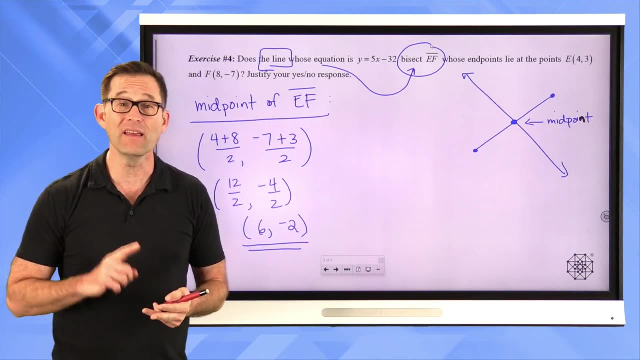 All right. So I know, I know that the midpoint of segment EF is 6 comma negative 2.. The question is: does this line pass through this point? Well, think about all the times in 8th grade math, algebra 1, and even a little bit in this course, that we've asked a question. 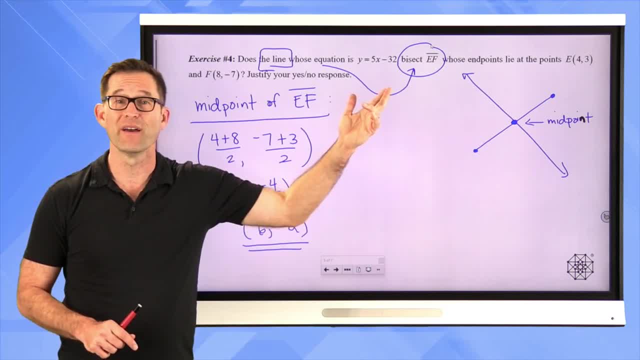 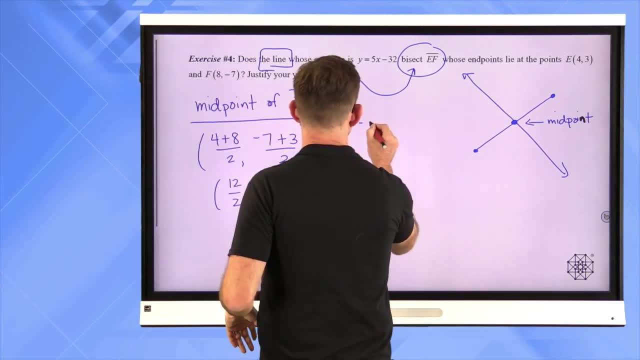 does this point lie on this line, right? Well, I can just check that. I want to see if this point lies on this line And to do that, I'm going to put negative 2 in for Y. I'm going to put 6 in for X. 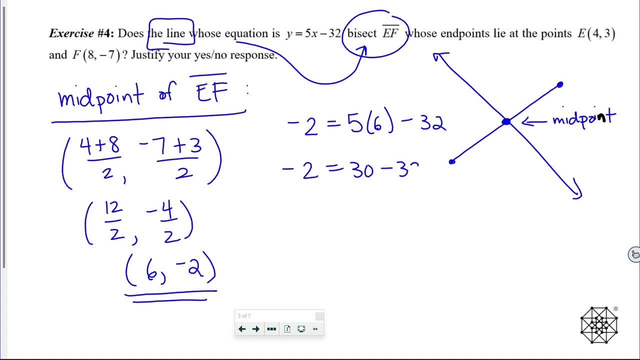 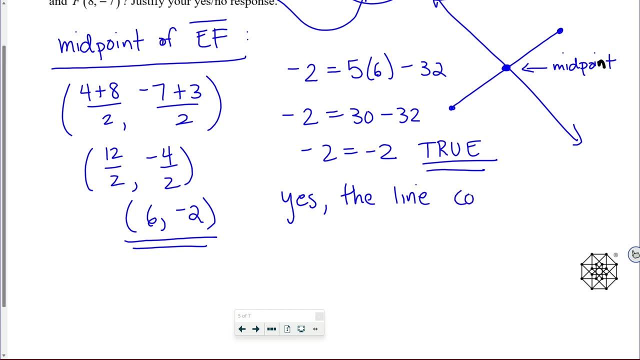 I'll get: negative 2 is equal to 30 minus 32.. Negative 2 equals negative 2.. That's true, And so the answer is yes. The line contains EF's midpoint, so bisects EF, right? That's the whole point. 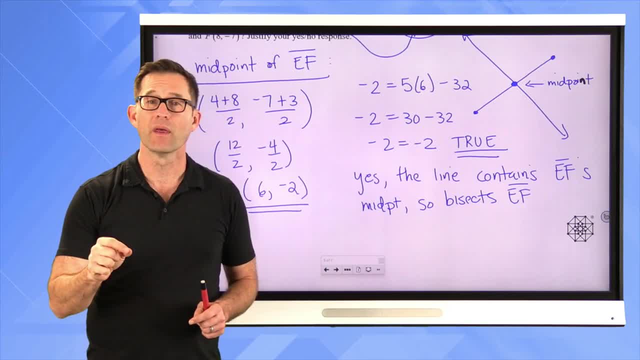 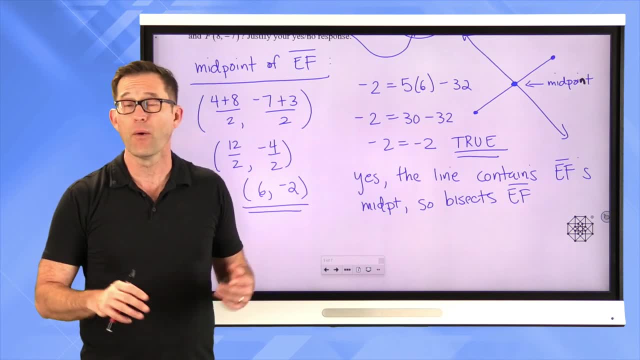 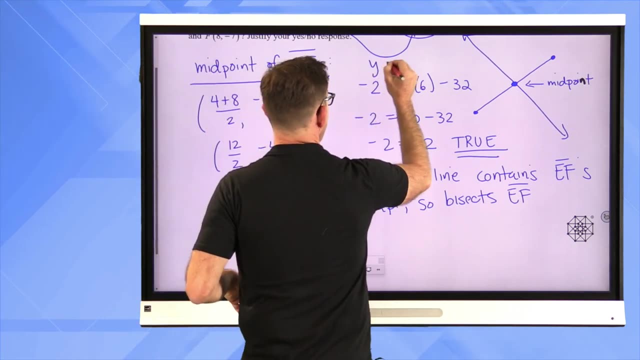 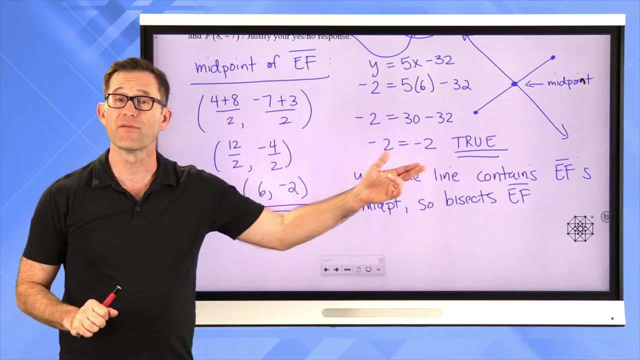 For a line to bisect a segment means for it to contain the segment's midpoint or to pass through the segment's midpoint, And we can tell whether a particular point lies on a particular equation or a particular line. In fact, maybe I'll put that equation right here by simply substituting the point into the equation of the line and seeing if it makes the equation true. 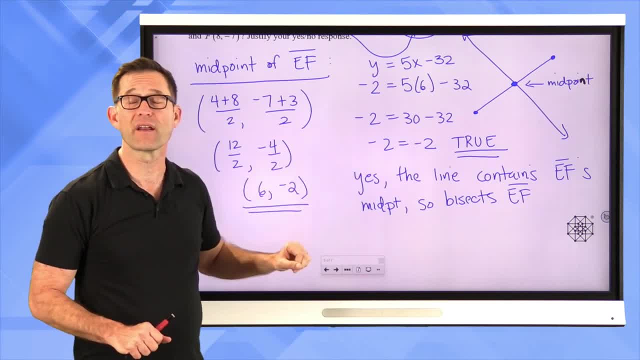 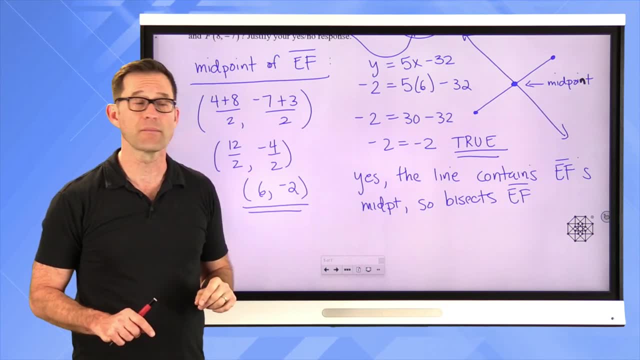 All right, Real cool. We don't need any coordinate grid or anything like that on here. Figure out what the midpoint is. See if it lies on the equation of the line. If so, the line bisects the segment. All right. 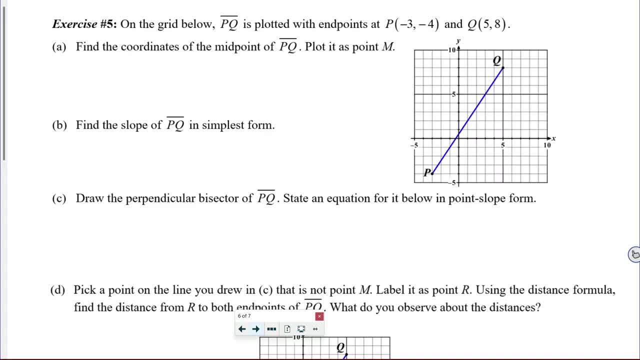 Let's take a look at one more, Exercise number 5.. On the grid below, segment PQ is plotted with endpoints at negative 3,, negative 4, and 5, 8.. Letter A: find the coordinates of the midpoint of PQ plotted as point M. 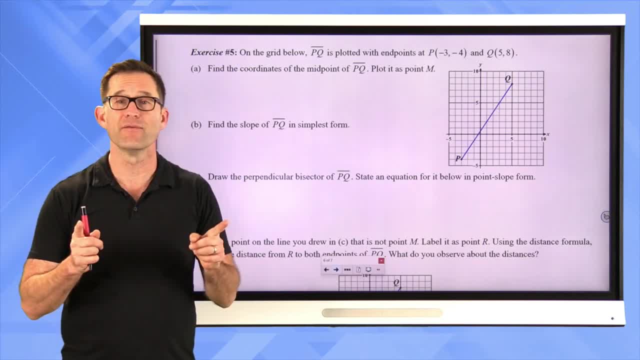 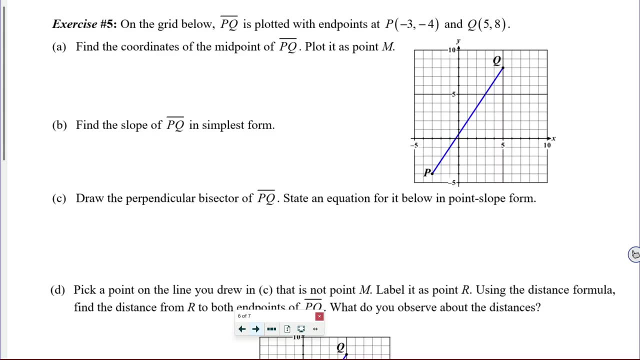 Awesome, No problem there. Why don't you pause the video now and go ahead and figure out the midpoint of segment PQ? All right, Let me do it. Here we go. So I've got negative 3 plus 5 divided by 2, comma: negative 4 plus 8 divided by 2.. 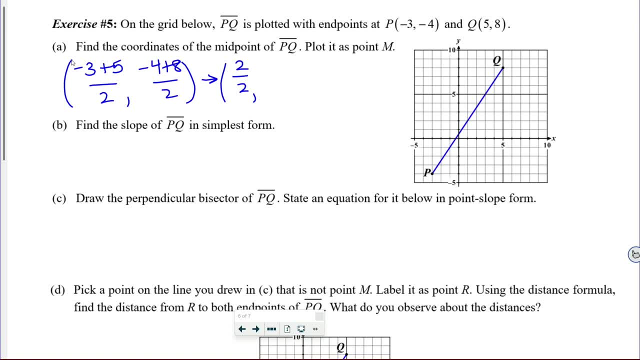 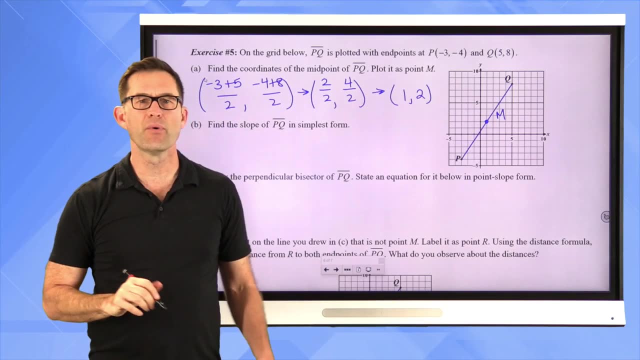 That's going to be 2 divided by 2 and 4 divided by 2, and that will be 1, 2.. That's a nice little midpoint there, So 1, 2.. Let me put it in right as point M for midpoint. 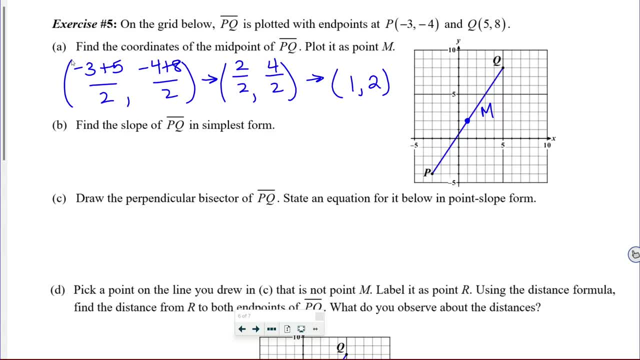 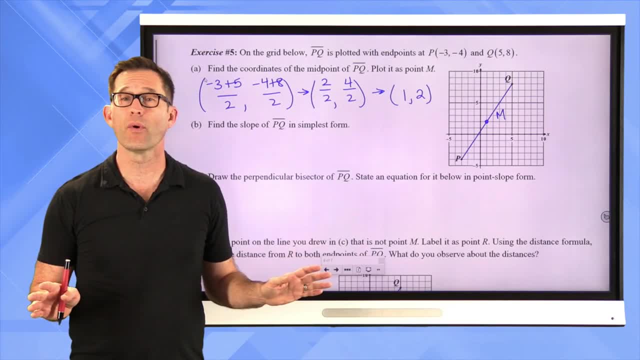 Awesome. All right, Let's take a look at letter B. Find the slope of PQ in simplest form- Awesome. So this has absolutely nothing to do with the midpoint right now. I just want you to find the slope of PQ in simplest form. 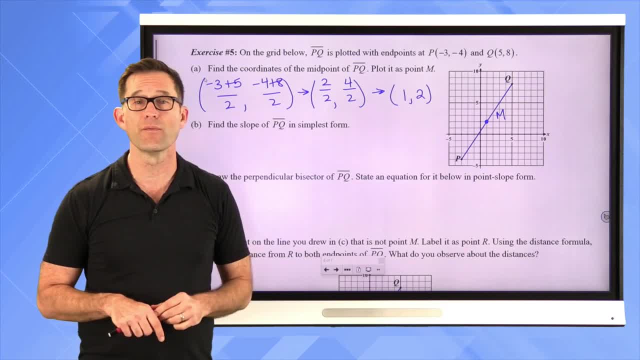 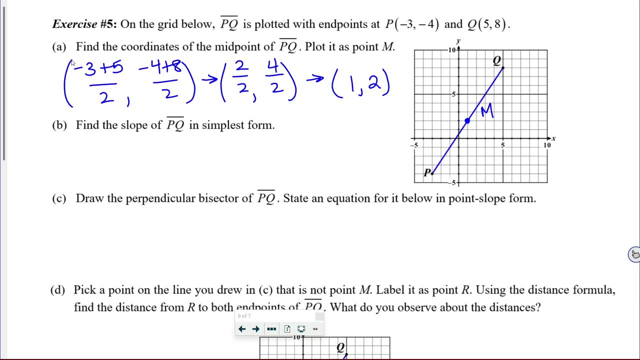 You could probably do it graphically, but you could also do it by using the slope formula. Either way, go ahead and find the slope of PQ. All right, I'm going to do it with the slope formula. It never hurts to see the slope formula again. 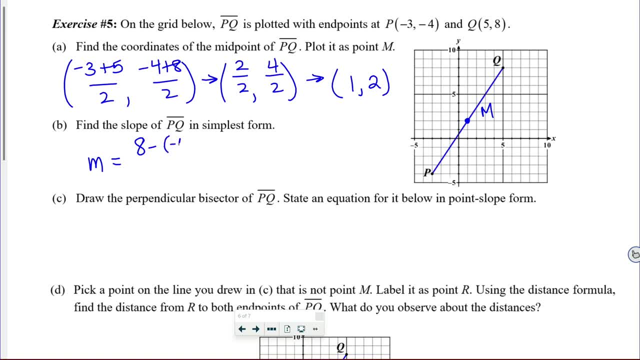 Right Slope is going to be Y2 minus Y1.. You just have to be a little bit careful there. Divided by X2 minus X1.. 8 minus negative, 4 is positive 12.. 5 minus negative, 3 is positive 8.. 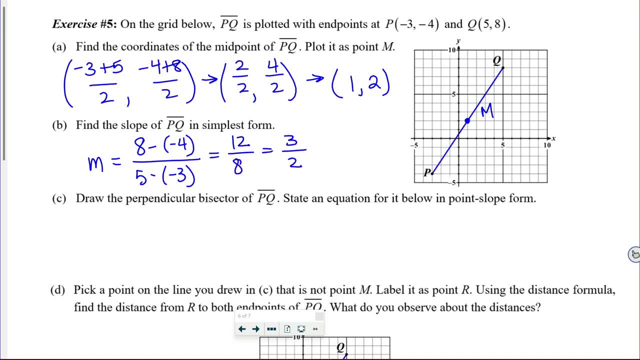 I can divide both of those by 4 and reduce my slope down to 3 halves- Awesome, All right, Let's take a look at letter C. Draw the perpendicular bisector of PQ. State an equation for it below in point slope form. 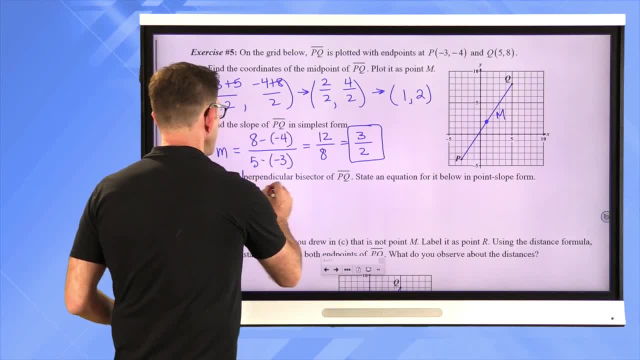 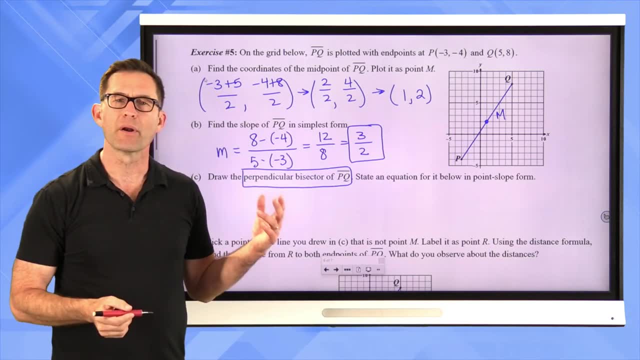 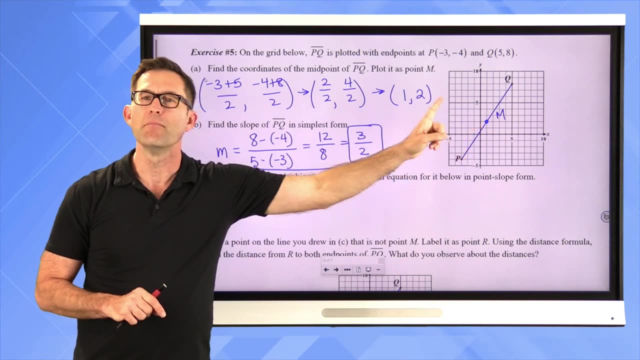 All right. Well, let's think about this just for a moment: The perpendicular bisector. Now, in the last problem we worked with a bisector, All right. But a perpendicular bisector is a little more special, right? Not only does it go through the midpoint, but it goes through the midpoint and is perpendicular. 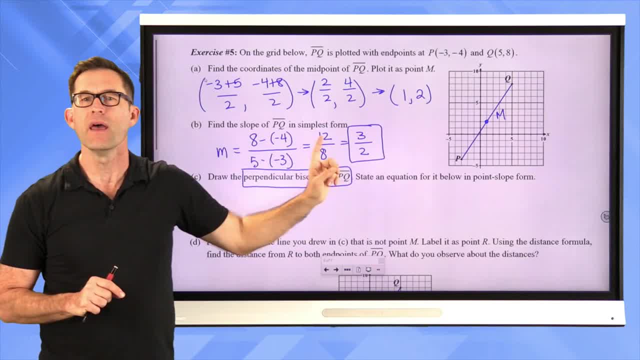 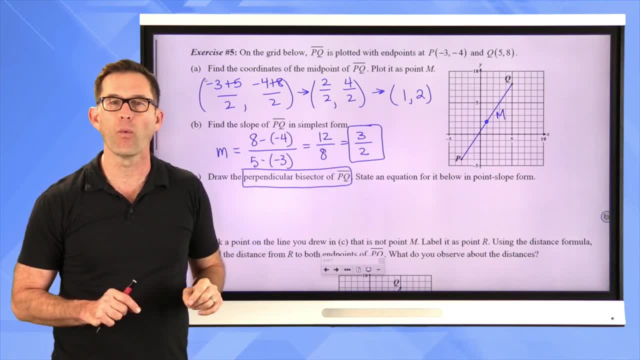 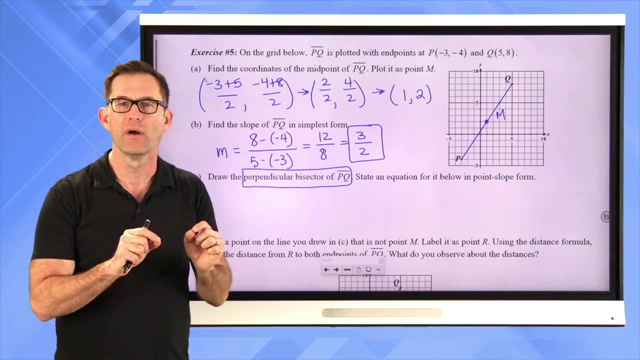 to the line segment in question. Now, I know that the line segment in question has a slope of three halves, So part of this is going to be to think about what the slope of the perpendicular bisector is. Pause the video now and, by thinking about that slope, try to draw the perpendicular 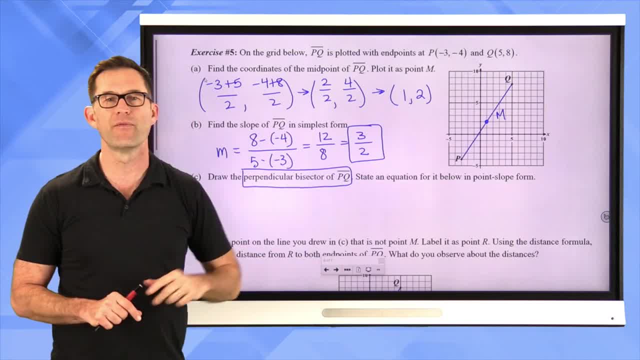 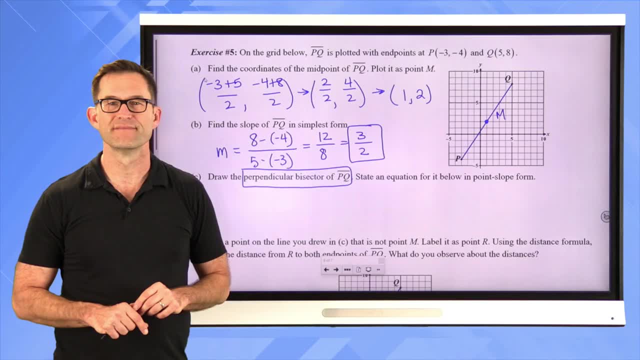 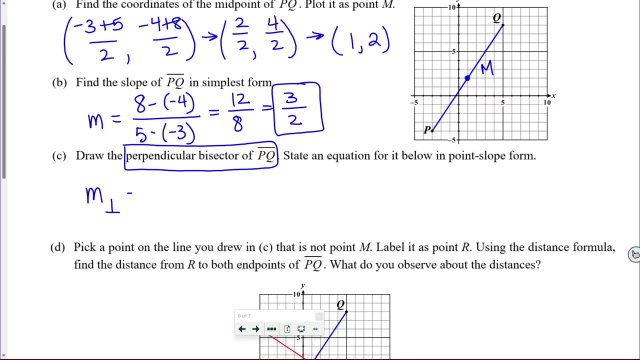 bisector, and then we'll come back and we'll talk about the point-slope form of its equation. All right, well, the slope of the perpendicular bisector. now I'll put it down as slope perpendicular must be negative, two-thirds right. So we're going. 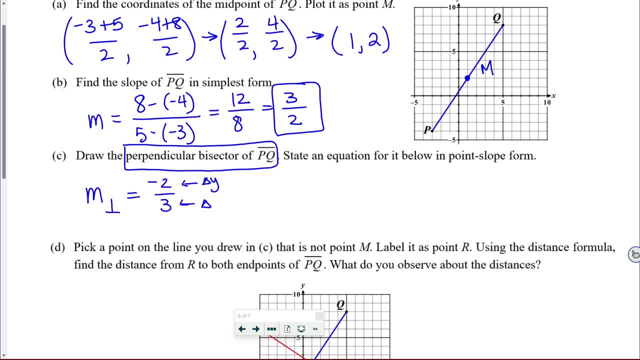 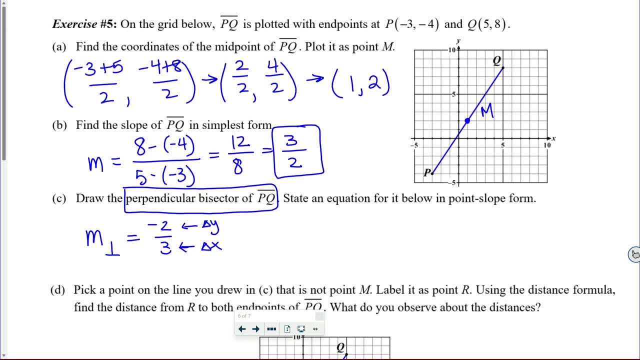 to want a change in y of negative 2 for a change in x of positive 3. That looks a little bit better. That will allow me now to go three units to the right and two units down. Three units to the right and two units down, and then I can go backwards and I 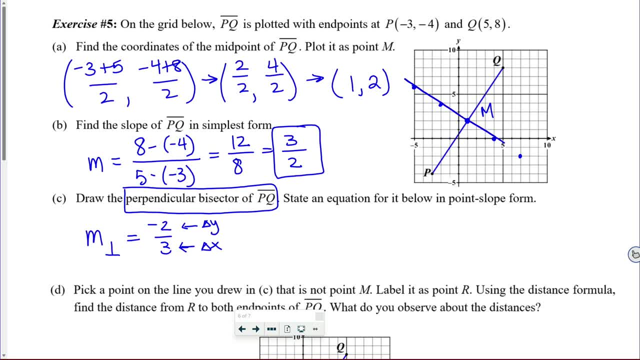 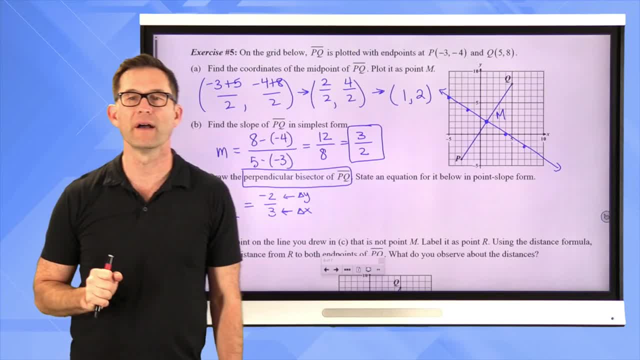 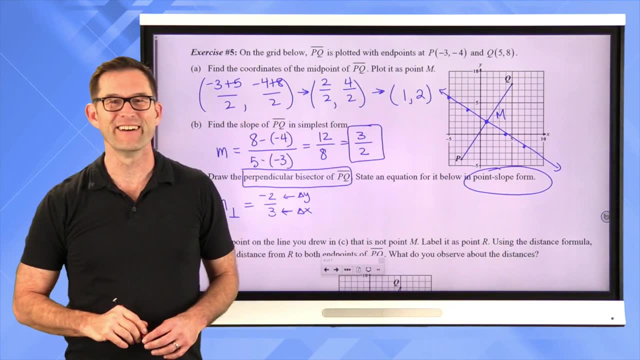 really should have my ruler here, but I don't. I'm just going to do that. That's not too bad. All right, there's my perpendicular bisector. Now I'd like to write its equation in point-slope form: right, This was something that was brand new to us. 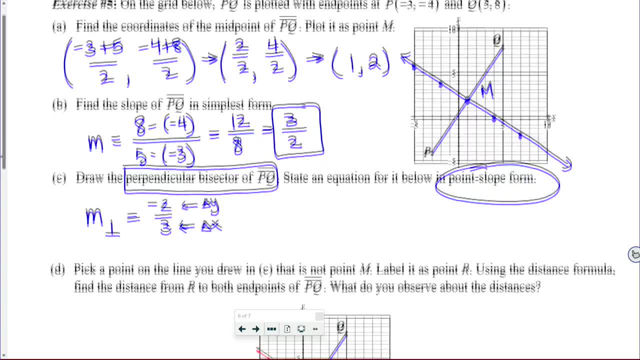 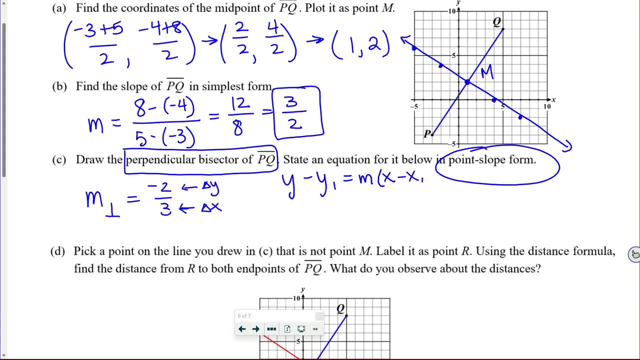 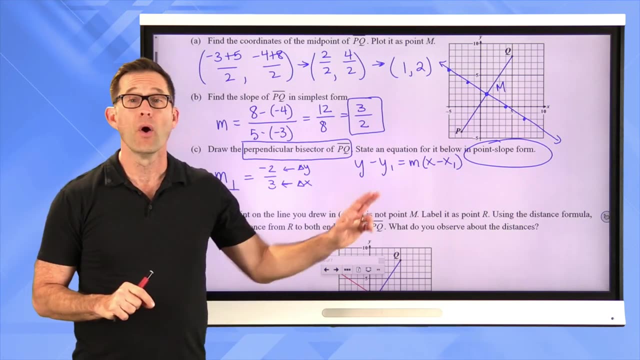 just a few lessons ago, Remember. point-slope form basically says: look, if I have the slope and any point that lies on a line, I can write the equation of it as: y minus y1 equals m times x minus x1, right, Where m is the. 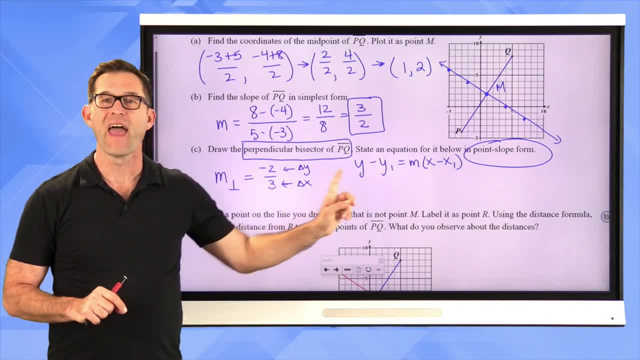 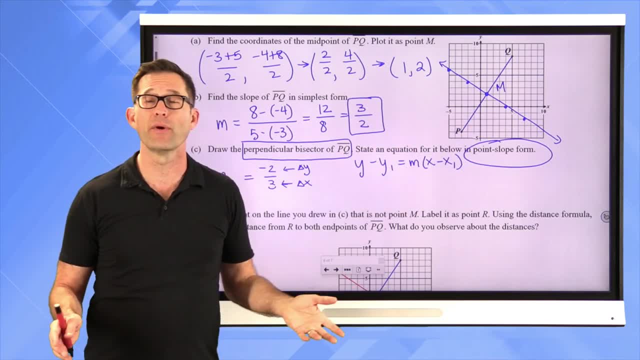 slope of the line which is sitting right here, and x1, y1 is any point that lies on the line. Now, granted, just by plotting this line, I saw lots of different points that lie on it, but one point that might be very convenient to use would be just: 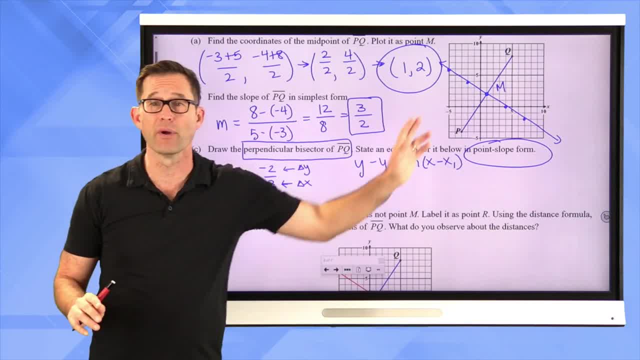 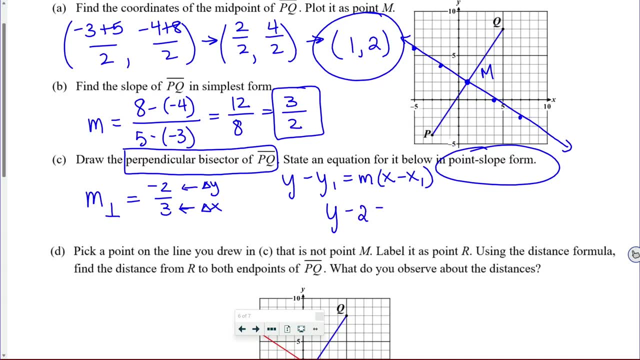 the midpoint And again, you don't have to use that point. Any one of the points I just plotted you could use, but I think I'm going to use that one and therefore I will have: y minus 2 equals negative two-thirds times x minus 1.. Again, any 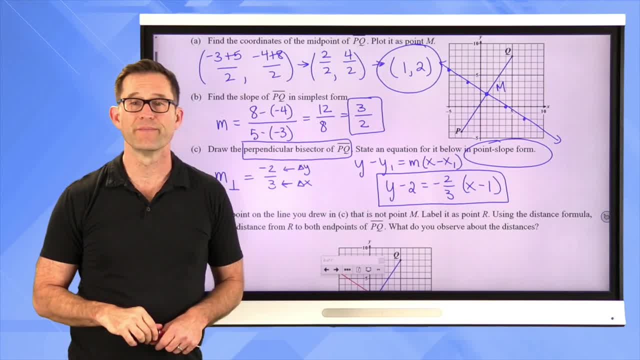 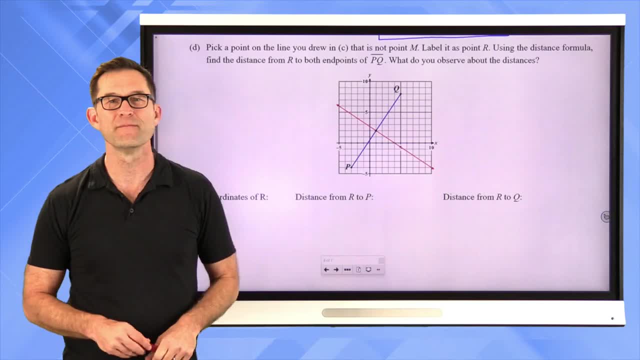 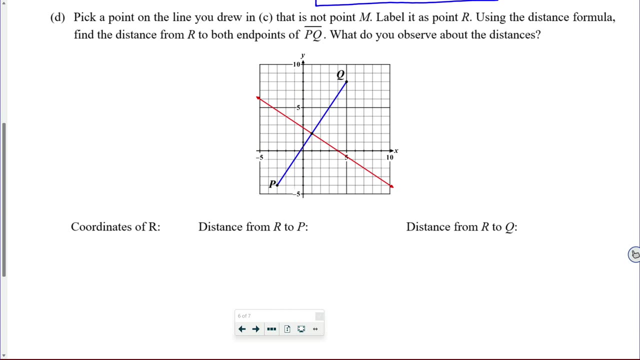 point could be used, though, that the perpendicular bisector goes through. All right, let's take a look at one last little piece of this problem and of this lesson. letter D: Pick a point on the line you drew in C, that is not point m. Label it as point r. 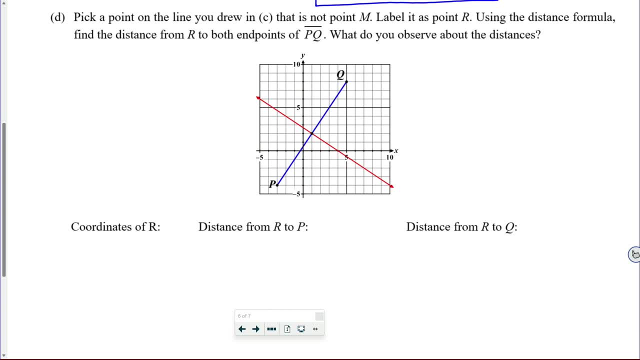 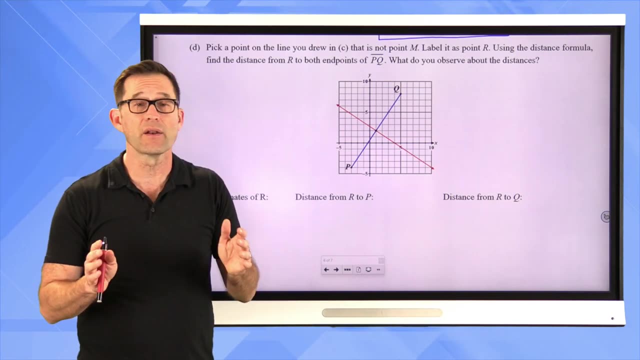 Using the distance formula, find the distance from r to both endpoints of PQ. What do you observe about the distances? Now, what I love doing with this problem, when I'm teaching it in front of a class of many students, is I literally say: pick any point along the perpendicular bisector. 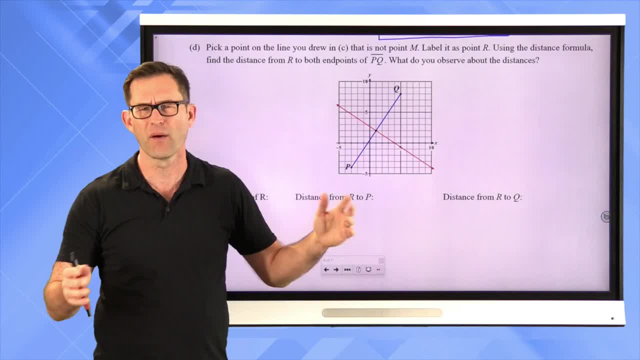 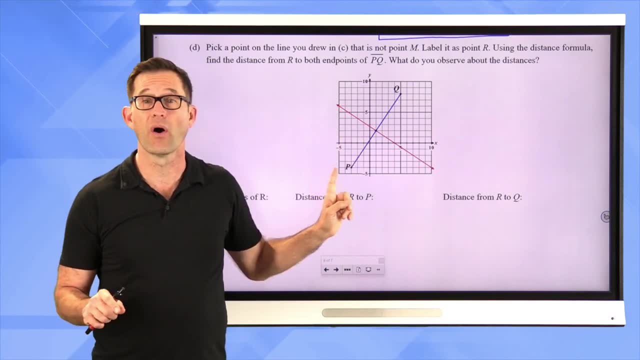 That's the one in red. now, right, Any point at all. You know, make it one of the nicer points, right, Just not the midpoint, And then, using that point, find the distance from that point to r, or, sorry, that distance from. 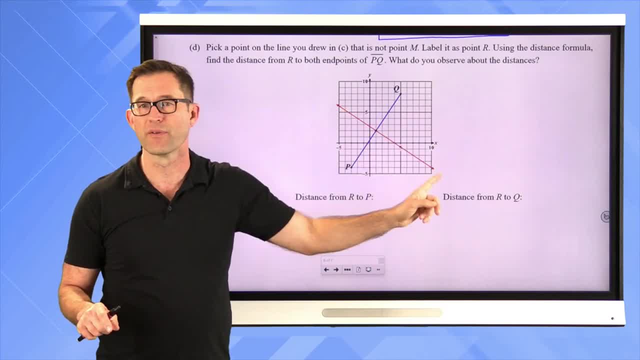 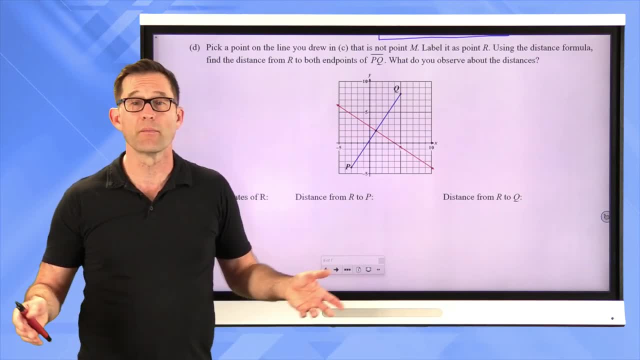 that point to P and the distance from that point to Q, or if the point's down here, right, And then kind of compare them all. right, Here we probably just want to use one particular point. So I'm going to- I think I'm going to go here, I'm going to. 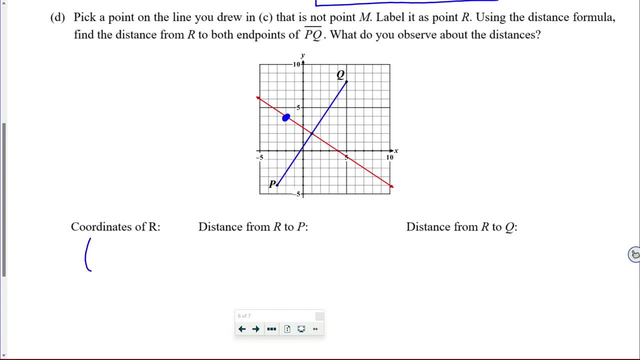 use this particular point, That is, the coordinates: negative two comma four. Now again, you could use that point. You could use the point negative five comma six, Four comma zero. would work great, Let's see. that would be seven comma negative two. ten comma negative four. Any of those points, any of. 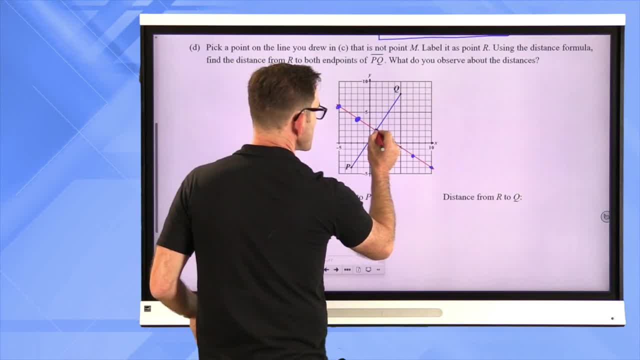 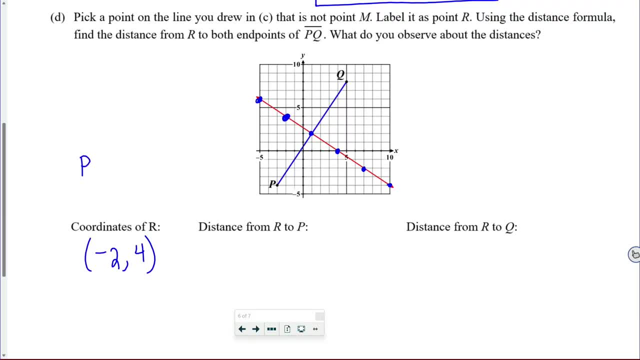 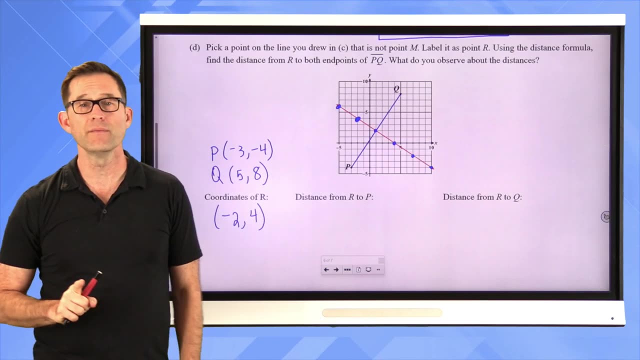 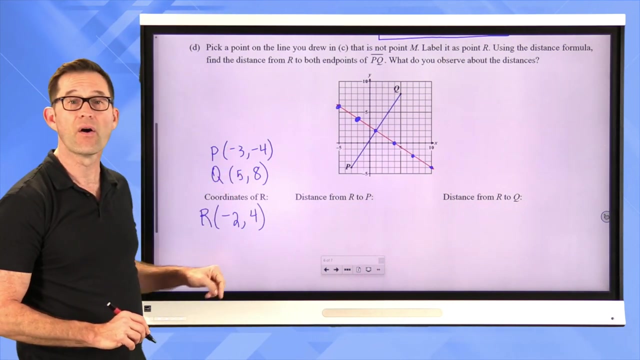 the two coordinates down: P is at negative three, negative four, and Q is at five comma eight. All right, What I'd like you to do now is I'd like you to find the distance from R to P and also find the distance from R to Q. Pause the. 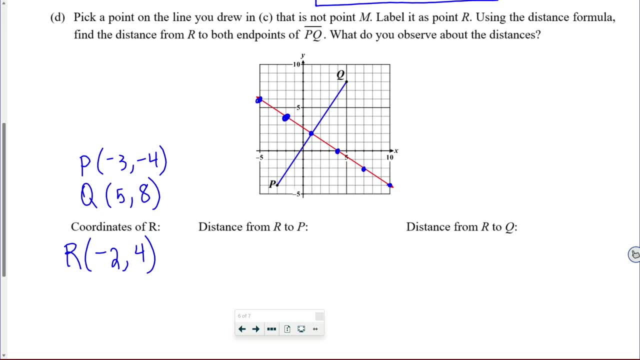 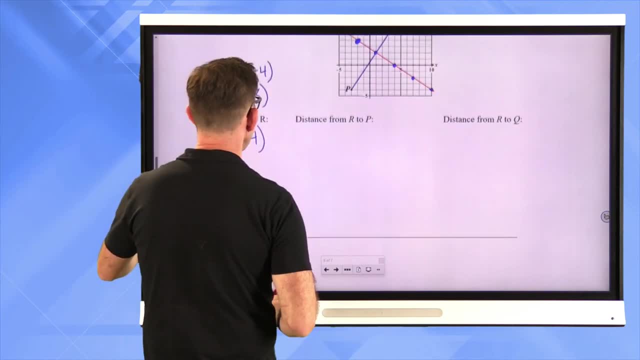 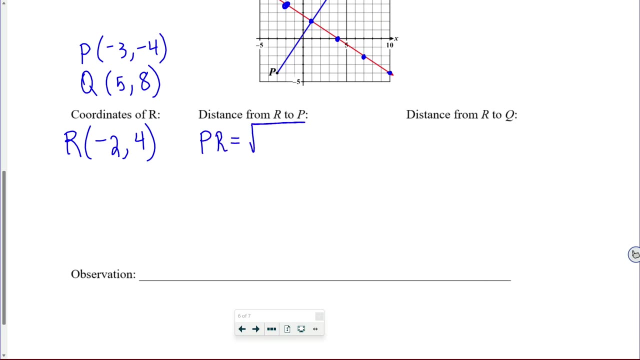 video now and go ahead and do that All right Time to do our distance formula. Here we go From R to P, okay, and I'll call this PR right. So it's the length of that segment From R to P we can. 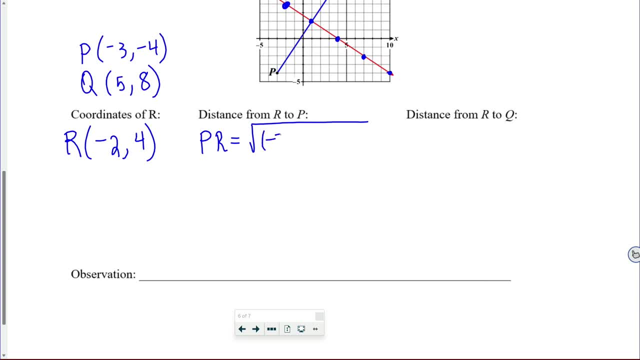 do the subtraction in either order. I'm going to do negative three minus negative two squared plus four minus negative four. All right, So I'm going to do the number four squared. lots of negatives there. Maybe I should have picked a different one. 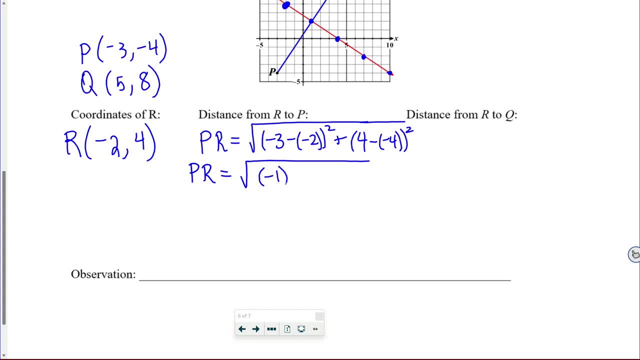 All right. Negative three minus negative. two is negative one. Just being careful, Four minus negative four is eight squared. All right. One squared negative. one squared is one. Eight squared is 64.. So I get the square root of 65.. Nothing really interesting about. 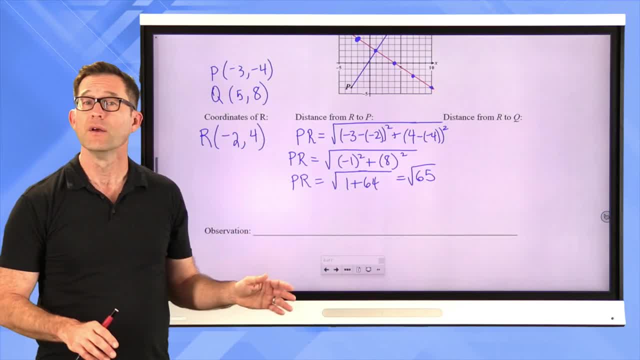 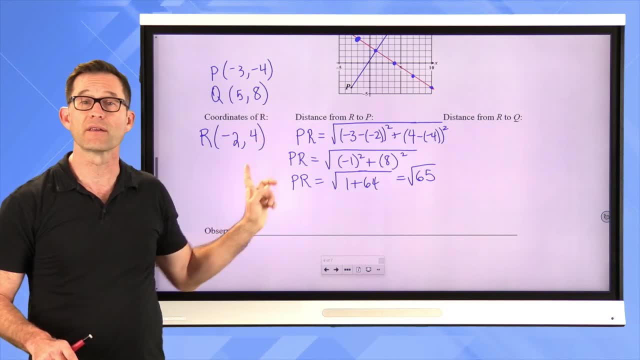 that. I'm not going to simplify it, I'm not going to put it in terms of decimal whatever. So the length of the segment that would connect P to R is the square root of 65.. Now we want to find the length of the segment that would connect Q to R. I'll call that. 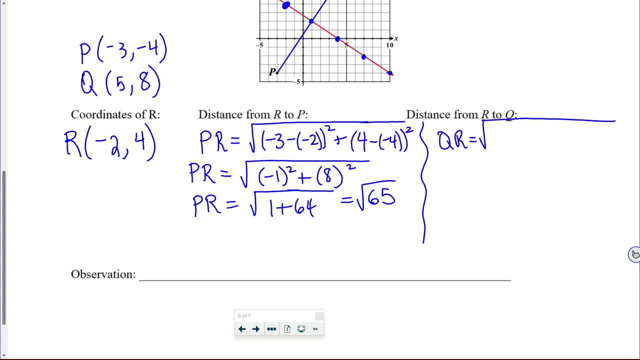 QR because it is. I have to write a little bit smaller here, but I think I can get it in there. So for R I'm going to have 5 minus negative 2, squared plus 8 minus 4, squared 5 minus. 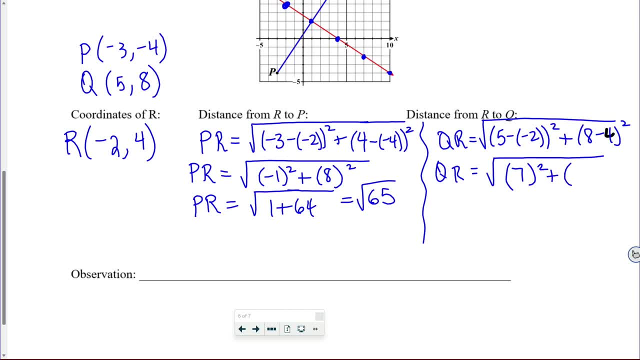 negative: 2 is 7, squared 8 minus 4 is 4, squared 7 squared is 49,. 4 squared is 16,. 49 plus 16 is 65.. And QR is the square root of 65.. 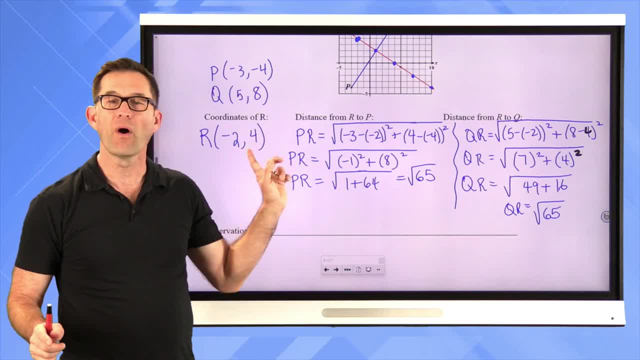 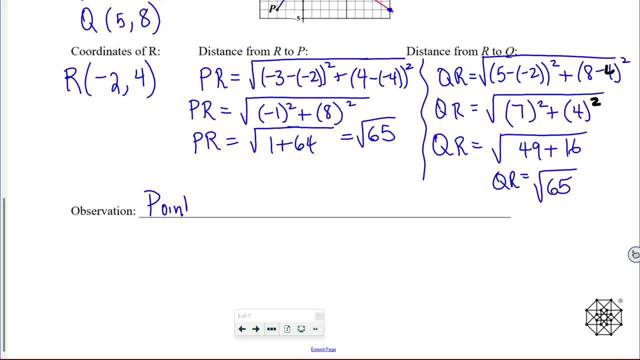 What observation can we make right? Point R is equidistant from point P and Q, And we knew that already, Or we should have. In other words, many times in this course, maybe even too many to count, although for a mathematician. 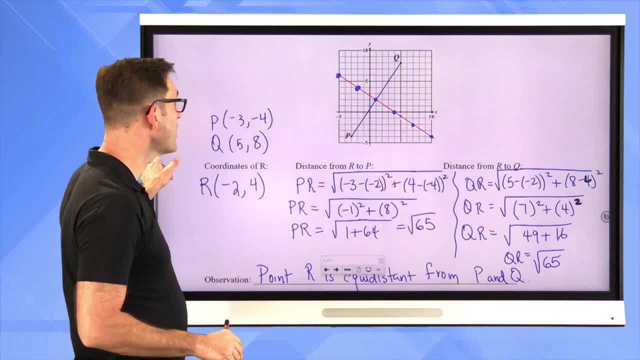 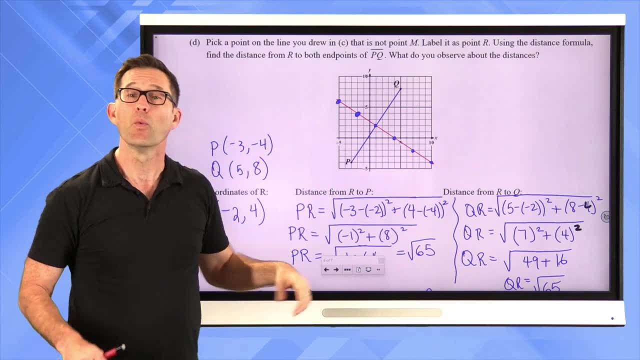 there's almost nothing. that's too many to count right. But many times in this course we've talked about the fact that any point that lies along the perpendicular bisector of a segment will be equidistant from the endpoints of that segment. 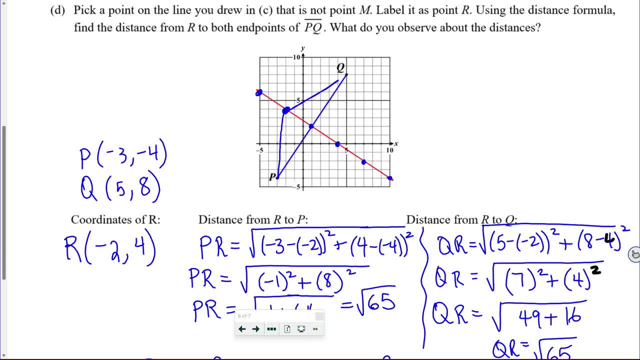 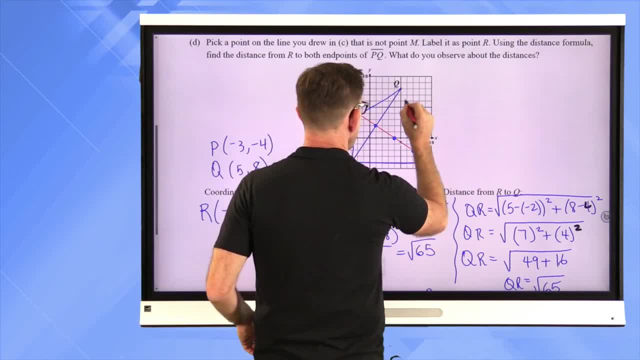 Now, literally what we just found is we found this length and this length And we found that those two lengths were equal. But if we had found, let's say, this length and this length, Those would have been equal, Or this length and this length. 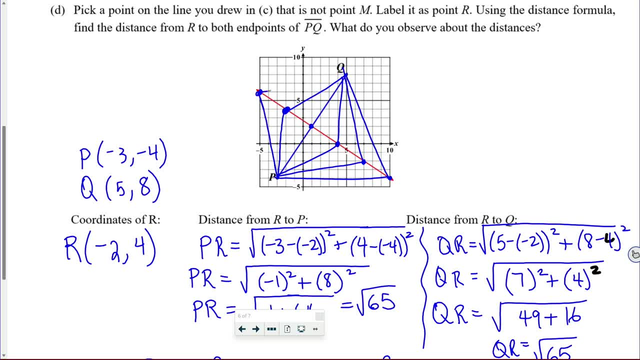 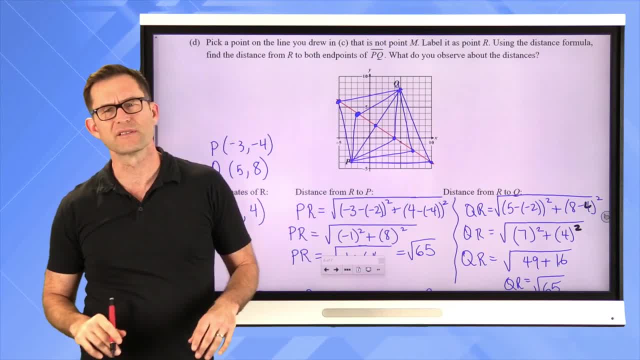 They would have been equal, Or this length and this length, et cetera, et cetera. all right, And really what you're getting is you're getting all of these little isosceles triangles. Granted, they're kind of like turned a little bit to the side and they give us a cool looking. 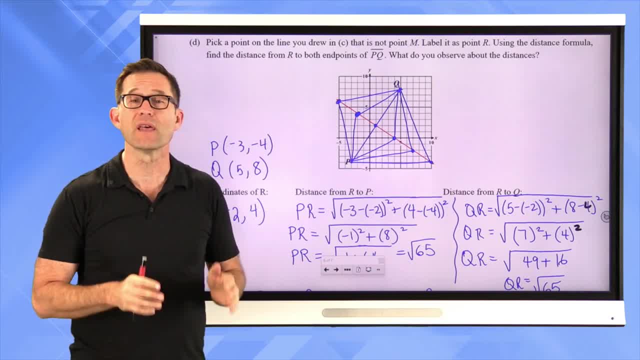 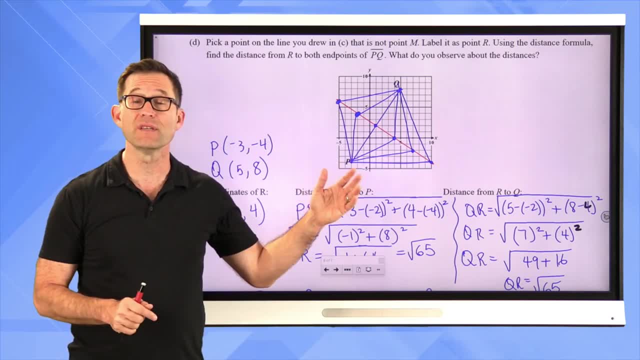 picture here. But one thing I just wanted to reiterate with this is that a result that we saw earlier- not in the coordinate plane- right in the Euclidean plane- we now see again in the coordinate plane And we can really verify it with things like this: 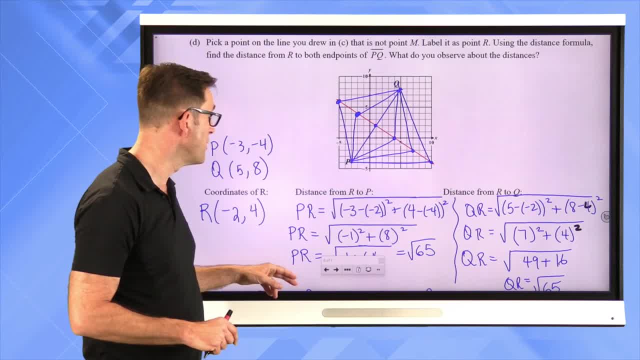 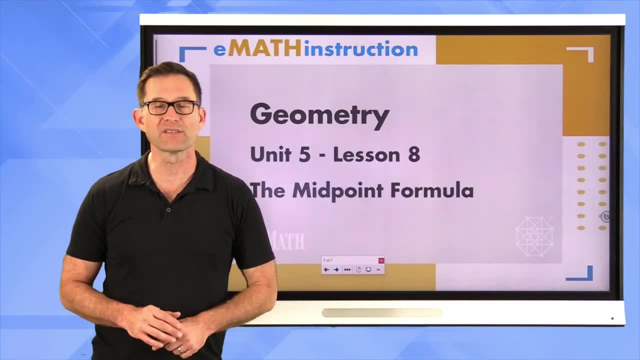 Things like the distance formula. This problem had almost nothing to do with the midpoint formula, except for the first problem, But it was pretty cool. All right, Let's wrap this up. So today we saw the last of our major coordinate geometry formulas.